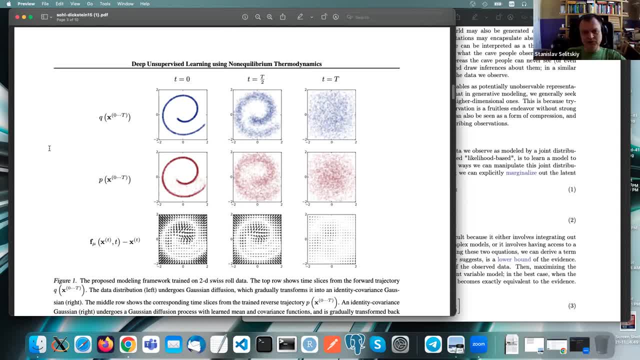 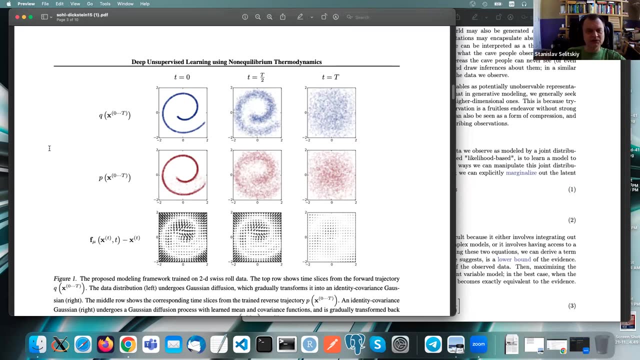 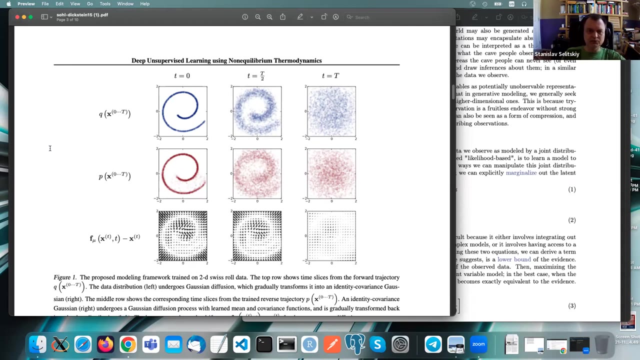 but using this diffusion mechanism Which is, on one hand, some kind of interesting and on another hand, I wouldn't expect it to like produce results, but apparently we have like quite interesting results And like basic idea of this autoencoder is to. so we have just two paths. 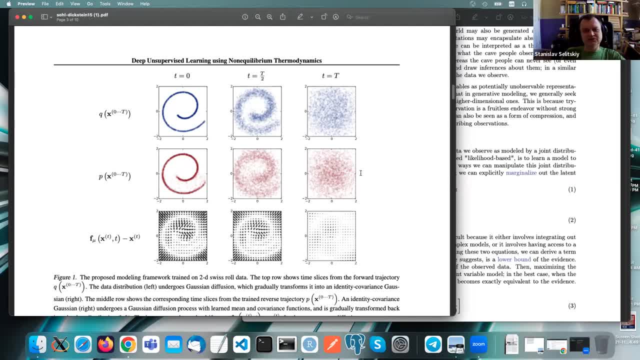 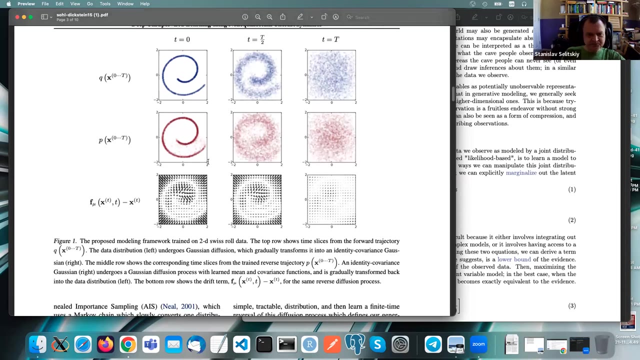 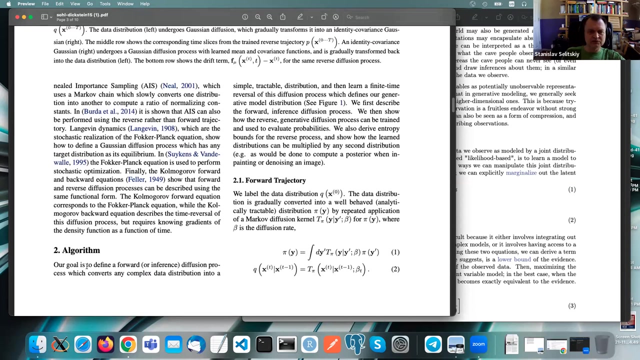 One is encoder and another is decoder And what we are encoding basically to the noise, And then we're trying to reconstruct, to decode noise back to something which has structure And they're talking about in terms of so, like you have like my description of Algaï. 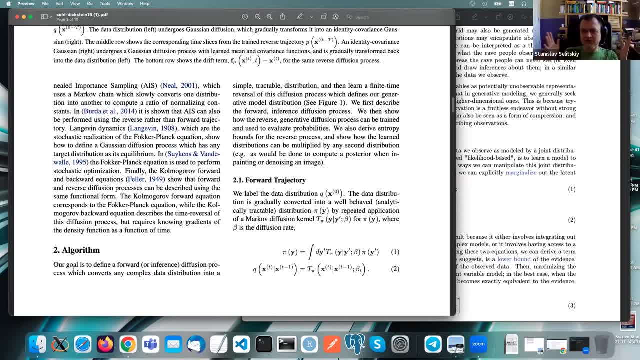 Yeah, Yeah, Yeah. algorithm where they say you have initial data set, for example, bunch of like. anything could be images, could be sounds, can be anything like text, and we like usually when we work with encoders, we collapse our dimensionality to something less than original one and thus trying to extract some kind of 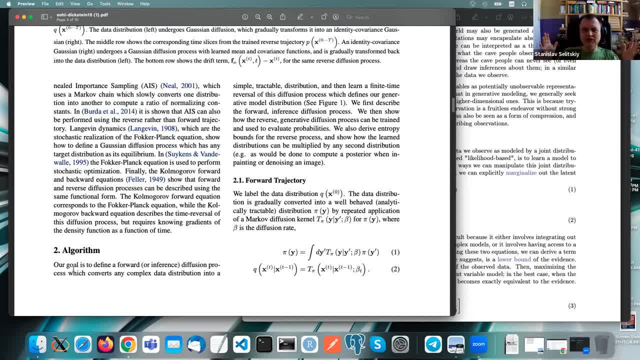 meaningful, like structure, here we encode to particle, because, like, we have some kind of non-parametric distribution of source data and then we like like we're not collapsing it, we like basically trying to map our distribution to some kind of a parametric distribution. in case of this paper they tried. 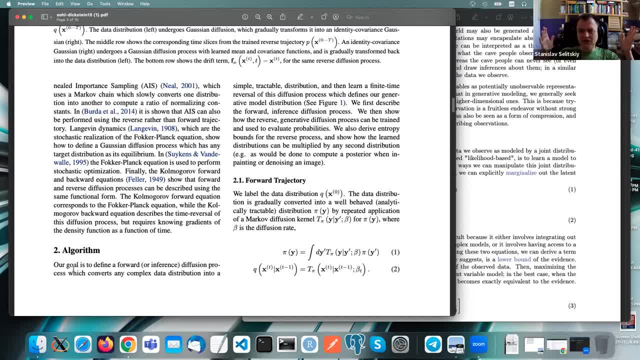 to once one Gaussian, another binomial, but I think it could be any parametric one and using again like stepwise diffusion to Gaussians. so you basically controllably increase our like chaos, like measure of our chaos. we corrupting, we're corrupting images to the distribution we like, which theoretically is tractable, and we use this like and also we. 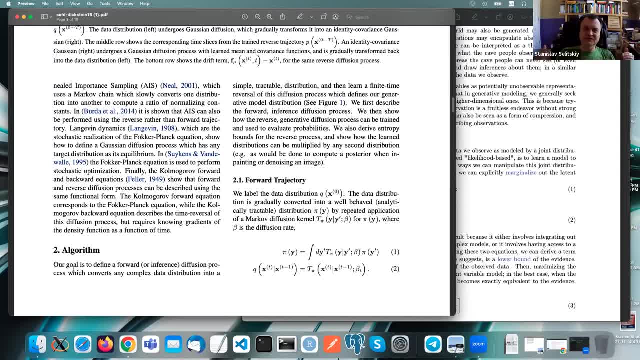 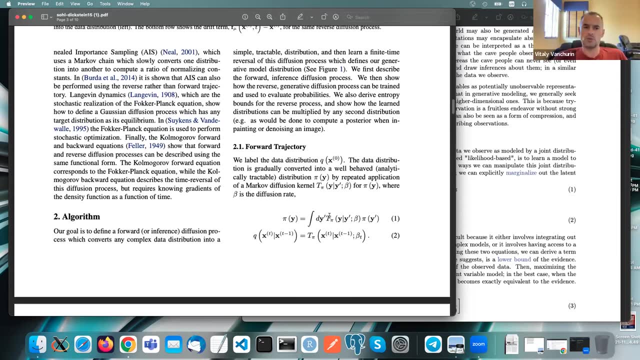 corrupting it, are using like theoretically tractable, again like Gaussians, we will use this later and so, yes, so this is so. so the thing is. my question is like, stepwise, let me I'm trying to understand the problem. setup so you have some kind of training data and then you're saying you're corrupting the training data, but do? 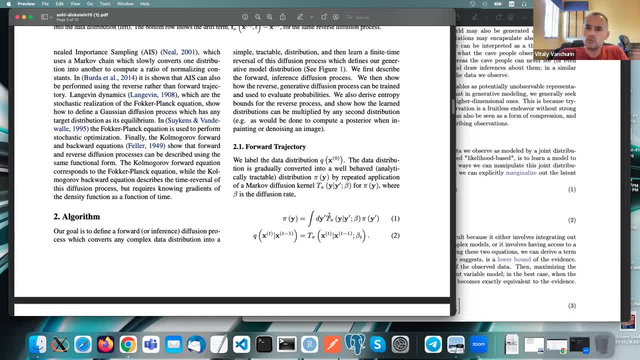 correct it and then, and then, once you corrupted that, then you train: yes, then, like, then we like train decoder, so, like, we corrupted this data on like very small steps. oh so you're saying the encoder itself is actually corrupting, nothing like this little superscripting. OK, we do це your ownơn, I just ordered it righticamente- and you correct it, something you're corrupting. and once you're corrupting, then you train: yeah, then then you create it again. oh, yes, so then you're saying: the en �edmo drive, we'll entrain them. so, look, we corrupted this data on a very small steps. spoilerote: we're corrupting Data on, However you know, a very small steps. 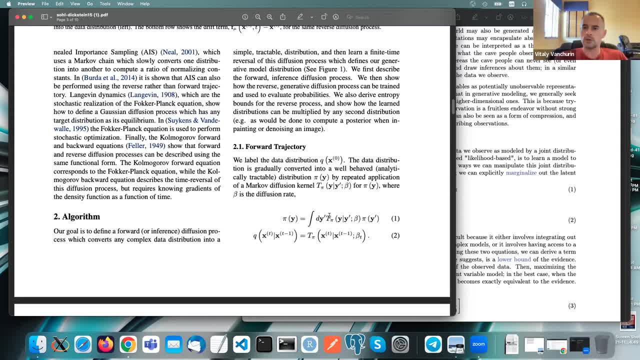 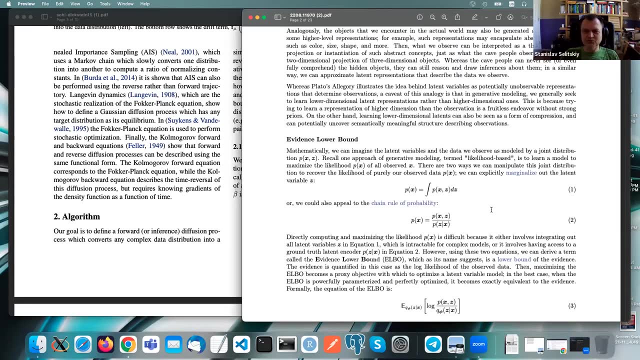 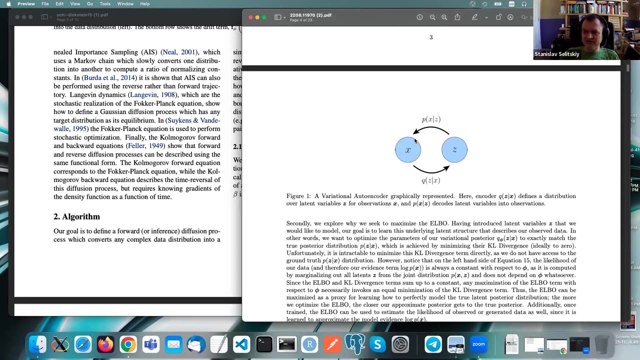 내 itself. is this corruption process or whatever? okay, yes, uh. and. and then you come to the bottleneck. or do you have a bottleneck there? uh, it's, yes, this is like bottleneck in terms of let me just show this paper. so we have, uh like simple, so we have x, we have our x like source data and bottlenecks. 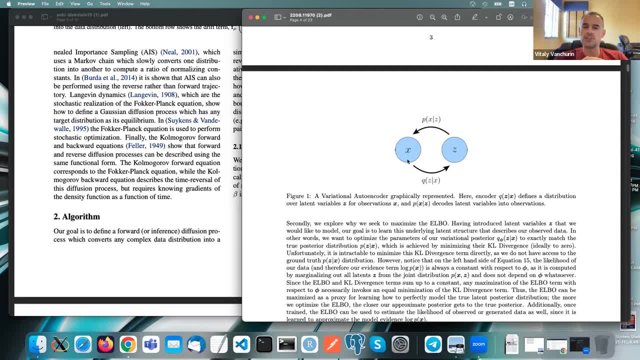 z, okay, and this process of going from x to z is what you're saying, the corruption, or whatever, adding the noise, yes, yes, adding the noise, or corruption, or, but that one is deterministic, it's not being learned, um, so we use, so, uh, they describe two approaches. one is we set. 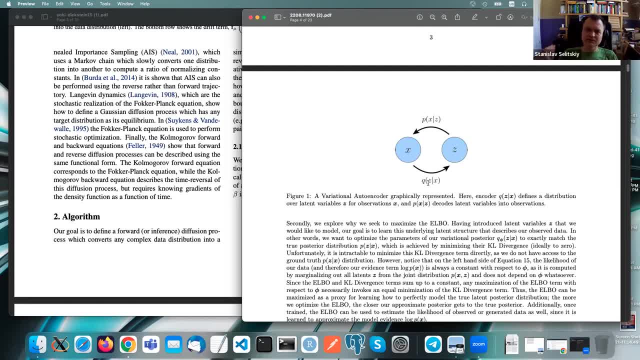 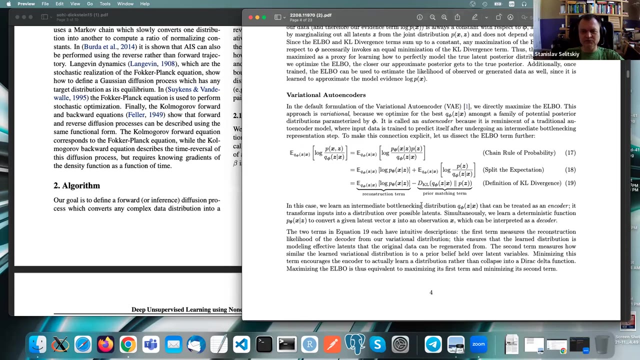 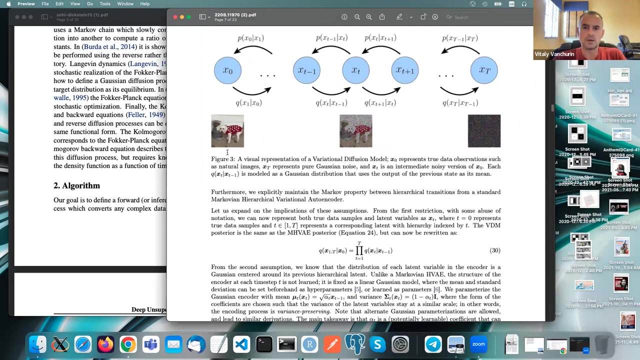 these parameters of diffusion, uh, as like hyper parameters or another or another modification, like learnable. so, okay, fine, okay. so then, then, uh, at z, you have some something completely diffused, right? yes, so we have uh diffusion, they also have this. let me go to some kind of illustration. yes, so we have. so we have original. 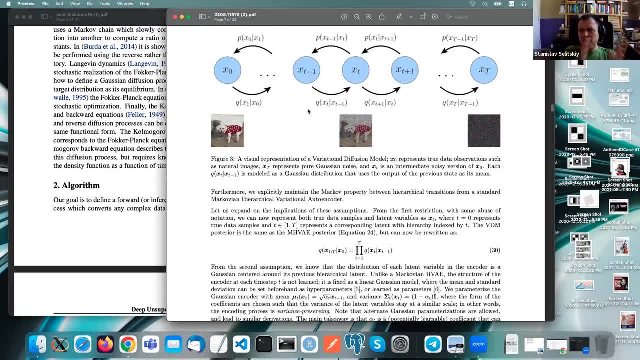 image, we on each. so we have multiple steps of corruption or adding the noise and finally we diffuse it to you know, like basically, uh, this, like normal, or like gaussian, where is z here? uh, here, like each next x is basically z. so this is like original, i see. i see, like this is like z1, z2, i see, and so the backwards arrow trying kind of. 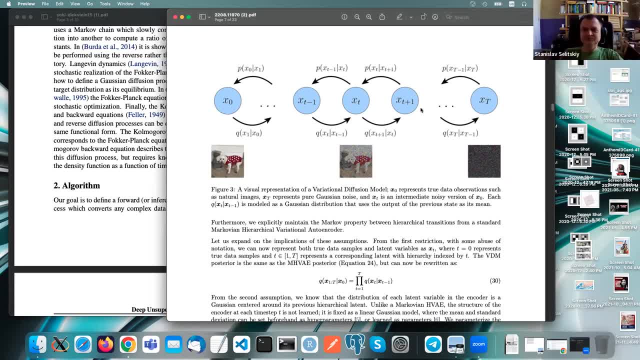 uh, undiffuse it, right, so yes, i see, i see. so so you're adding no noise one way and then trying to eliminate it the other way, right, i see? and by that we're learning, uh like structure of the um, like of the picture, like trying to controllably, uh like include noise and then, uh like remove this noise, reconstructing. 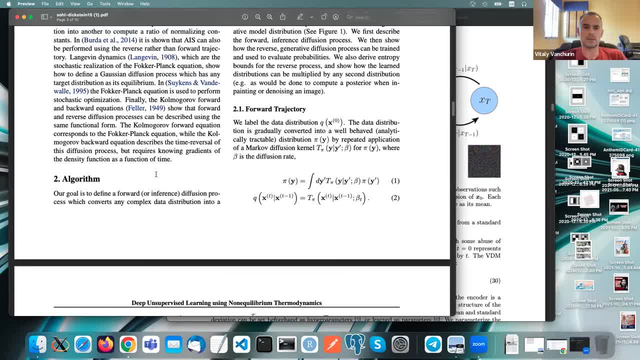 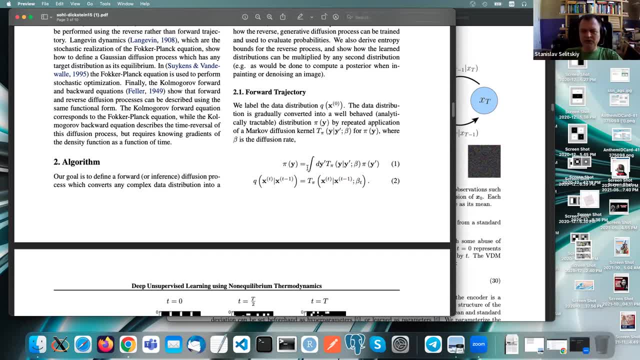 original one, right, and so they're talking. so here we have this like gaussian uh uh kernel and we basically using like previous uh they have little bit uh like different notation, but uh x is uh the same. here we have uh y like intermediate, but basically this is uh like saying: we have this chain of uh of of gaussian like corruption. 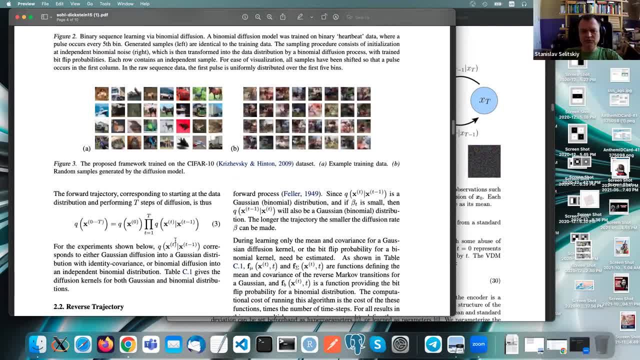 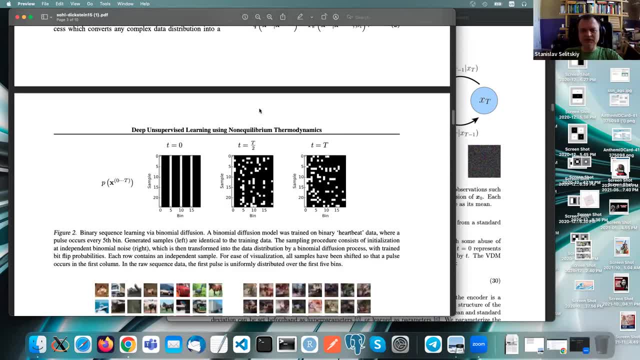 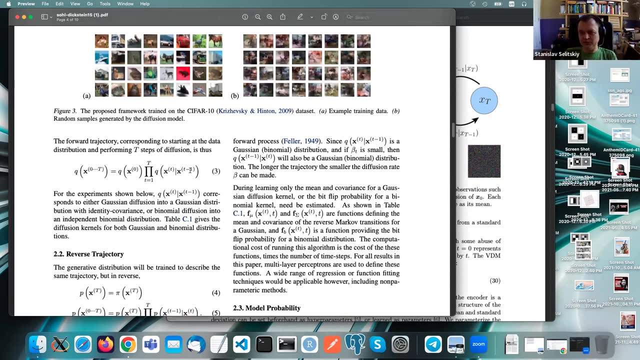 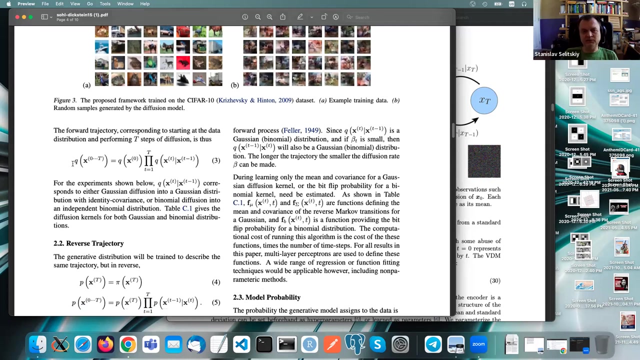 and uh, because we have so uh and they they describe like forward path, like forward uh trajectory of the data, so on, each, each step from x uh, a tab previews the current. we have our distribution and we go to the electrobic there and each time we um uh multiplicate uh these probability distributions and we get like you and 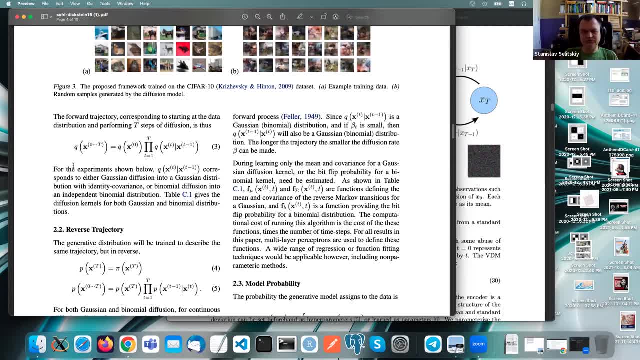 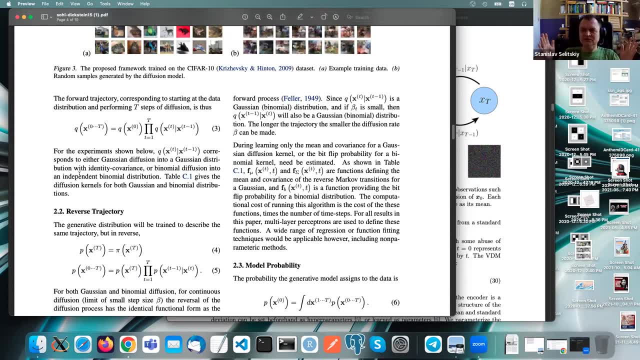 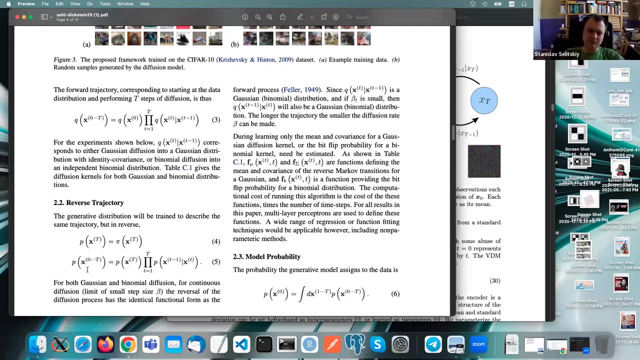 uh, uh. this is modeling distribution, and like modeling i mean like. so we have our like original, not parametric, like like really strange distribution and we're trying to squeeze it by adding noise into like noisy, uh like normal distribution and and p. this is uh like reverse pass. we're going through uh from our uh ideally. 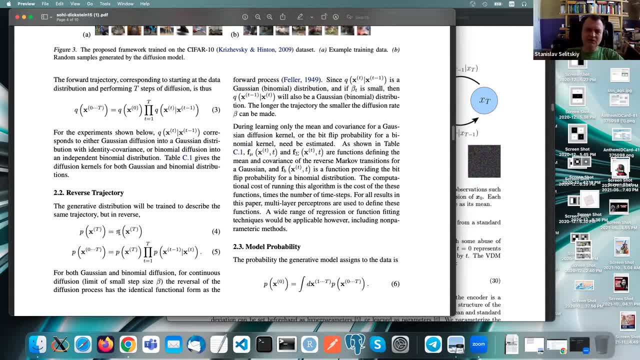 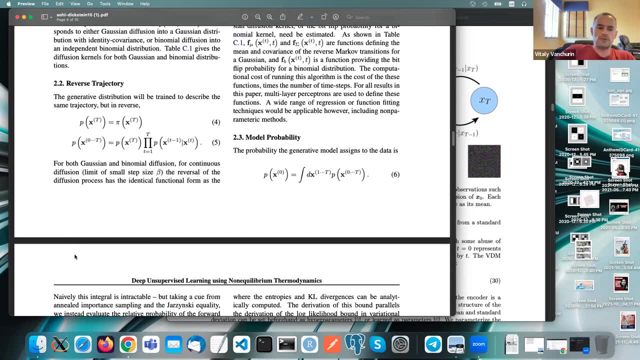 uh, like gaussian distribution, so like pure noise. uh, uh, back to our original, like original picture or text or whatever. uh and well, it's not pure noise. if you can reconstruct a picture from it, it cannot be a pure noise. so i think i'm still missing something there. yeah, so this is a. yeah, like this is high level and like 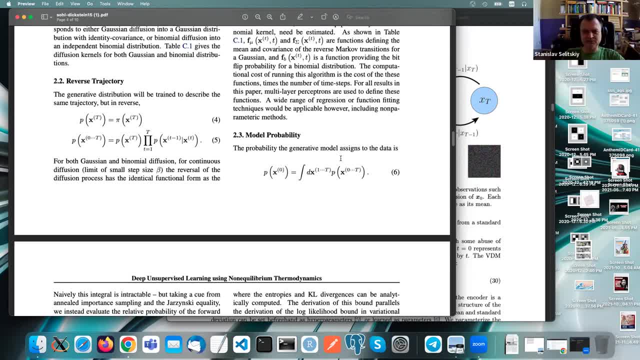 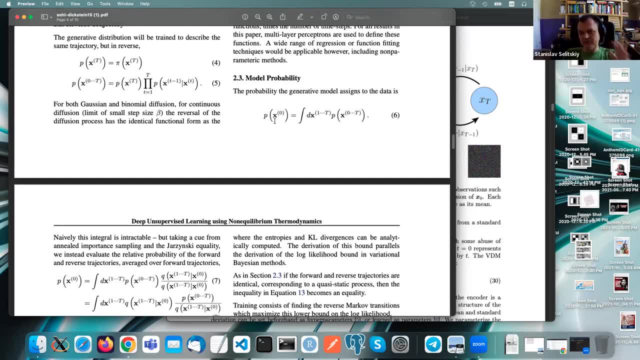 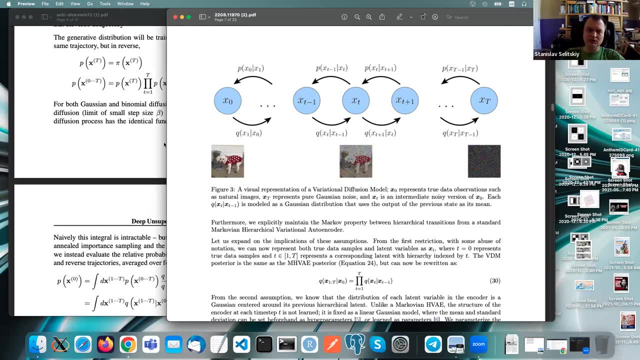 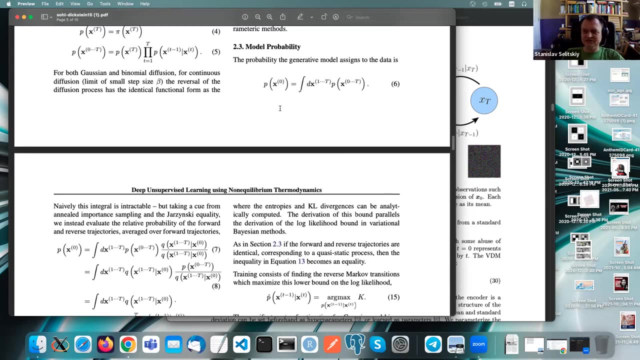 we go to the second uh to go like step by step. so they are like they starting with this probability of reconstruction of the like uh, final. so we uh like, get here, like from this noise we get here to original one and we have this probability. we want to maximize it in general settings is like really difficult, like 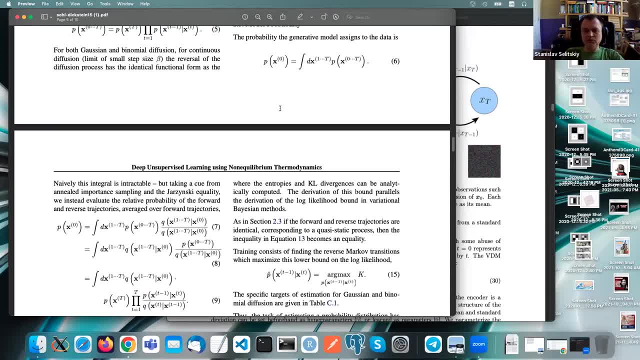 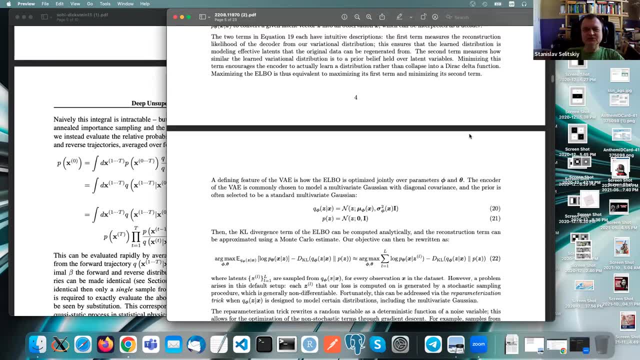 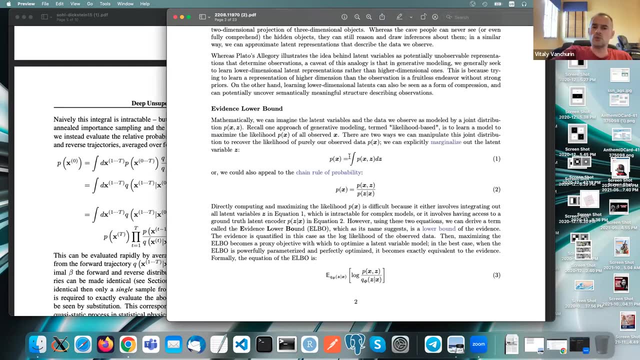 probably uh untractable. and here we do series of tricks which are, like, better explained here. so let's, let's go back to the original case. uh, so, uh, they like talking about, yes, sorry, and this q, uh, the transition matrix q, or whatever uh is, is uh the same for all steps, from zero to t right. 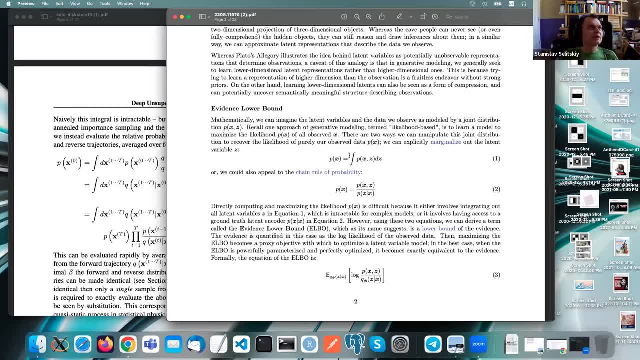 uh, that could be like different. so like: uh, no, q must be the same, it's just they use the same you know letter, so it might. and p has to be the same, like all the forward and reverse pass. uh, they're like. they're like encoder and decoder, right? yeah, so this like steps of of encoding and like and decoding, so we have. 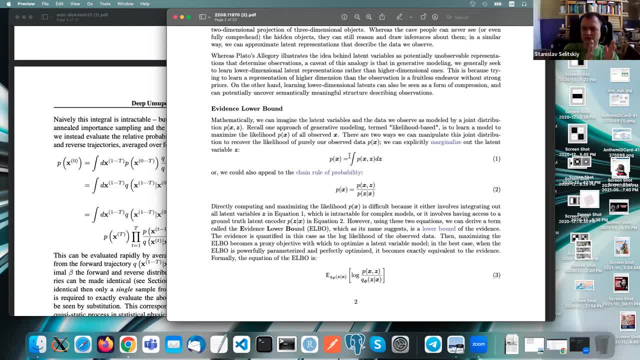 so we have like, for example, like you, uh, for the first step, uh, the same q for the second step, uh and yeah, so, like like for second, we, uh, we use first q as a source. so there's like uh like mark of steps. so we have no, no, i understand that you use uh output from the first step into the thing. 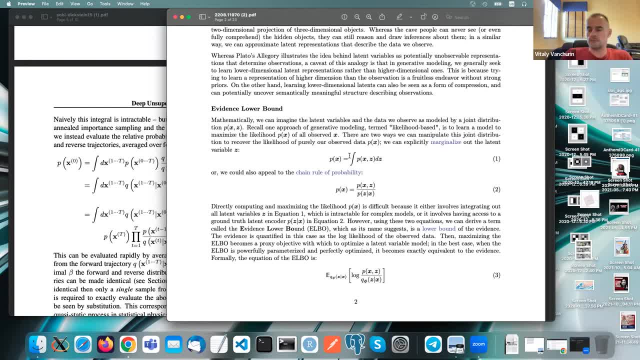 but the, the function q, uh is the same. this is conditional probability q um, it's just, it's, it's described by your neural network, by your encoder, yeah, so so, yes, uh, uh like. generally it could be different, but for this model this is the same. the difference is just, uh like, just parameters, right, uh like this diffusion parameter. so, 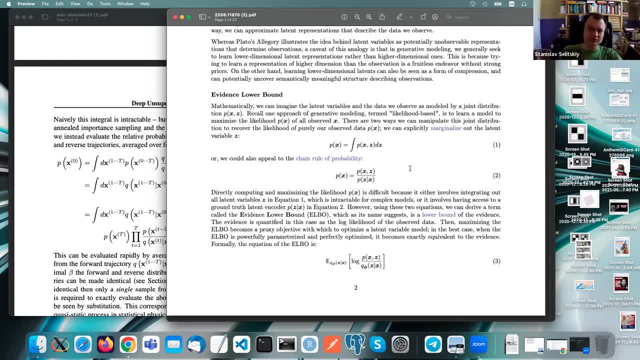 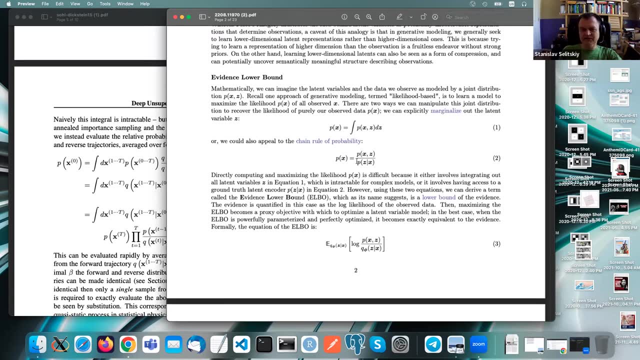 uh. they start with simple. so this is like second, more explanatory uh paper. they start with uh like simple, uh probability equation like this, uh marginalization of joint probability, and like chain rule and uh what they want, like where they want to go from there. this is a tool. uh like evidence, uh like 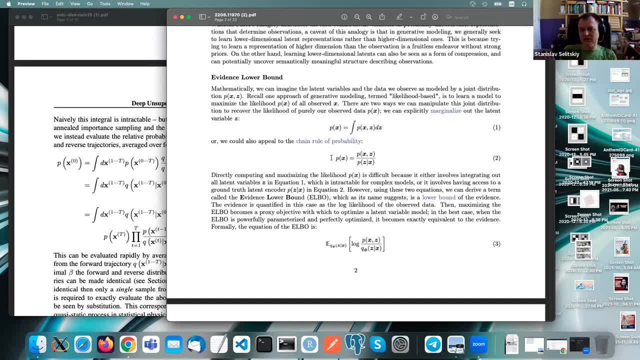 lower bound. so like we're talking uh this chain, uh probability, in context of uh bayesian equation, so this is some kind of left part we have uh like posterior uh p is that uh like conditional. x, x is like evidence and marginal distribution: right. marginal equals to joint divided by condition. 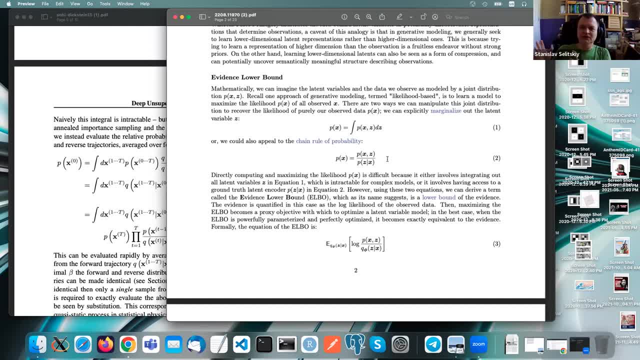 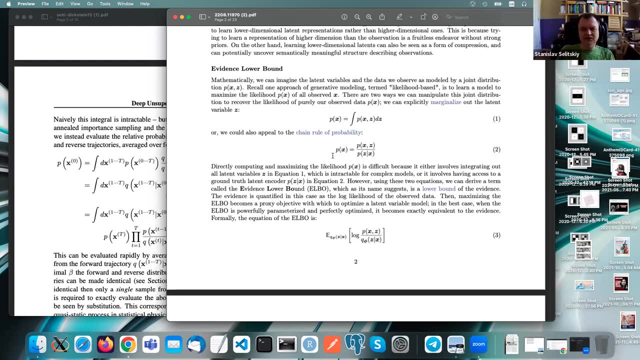 so like, uh like on other side we can have this: uh like pz, uh, uh like multiplied or like conditional px from z, but uh like, for starters, they use uh just one, uh, just one part, and they come in to use this, uh, evidence lower bound, uh like they. 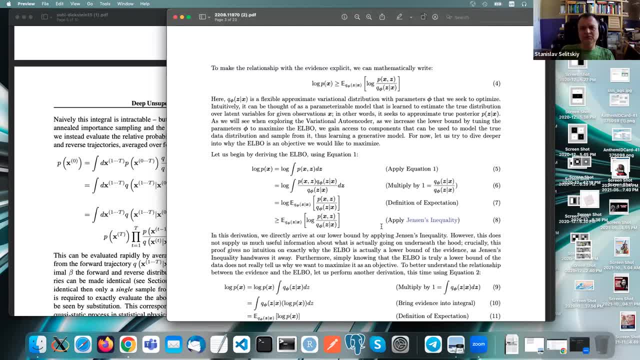 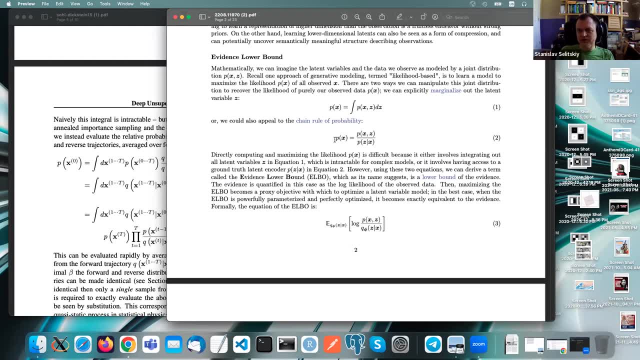 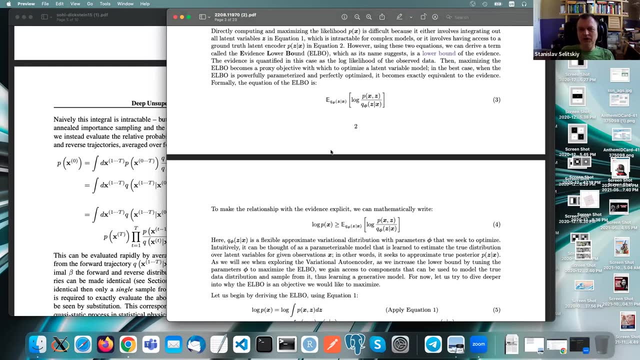 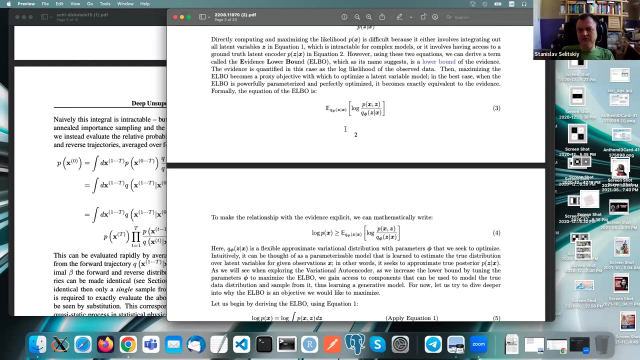 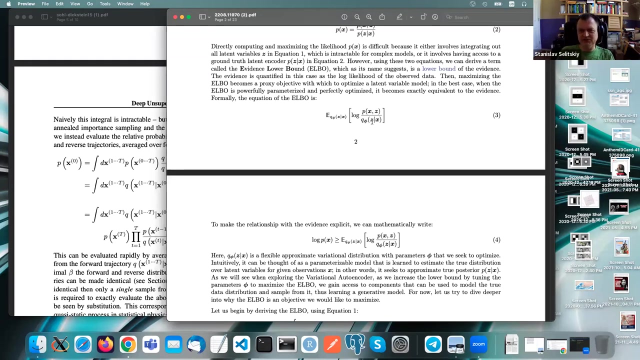 declare it here. but here they explain how they like: instead of optimizing uh this probability distribution, like uh this marginal x, they want to use uh for like optimization, actually for maximization, uh, this one lower bound. so basically, this is um, uh expected value of the lock of like this division of joint by uh with the conditional and here uh. 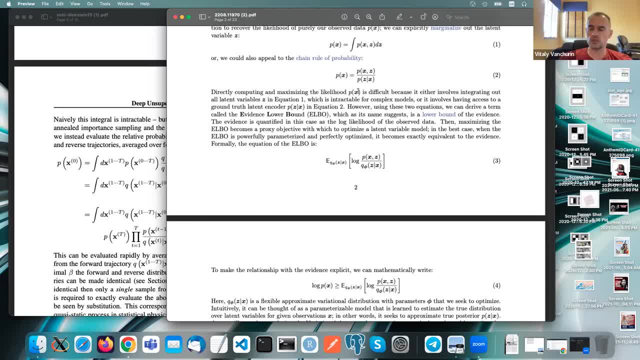 there is. basically, they're just saying that we want the two distributions to be as close to each other as possible. right so, the one that you started with and the one that you get on the uh. but we have also intermediate step. we also want, like a, like final one, uh, like a. 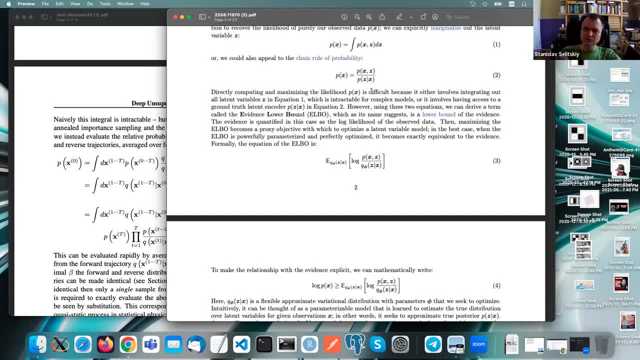 final one of the uh bottleneck, like supposed to be uh gaussian, like this one, uh, this, uh p like conditional z of x, z, this is like final z, so this z on the like bottleneck and uh, this supposed to be like true gaussian. and here is our q. in our model we try to get as close as 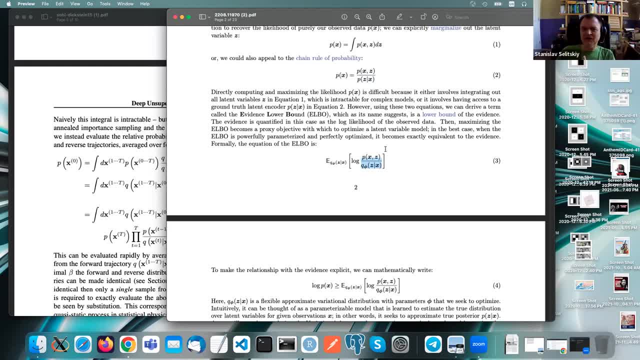 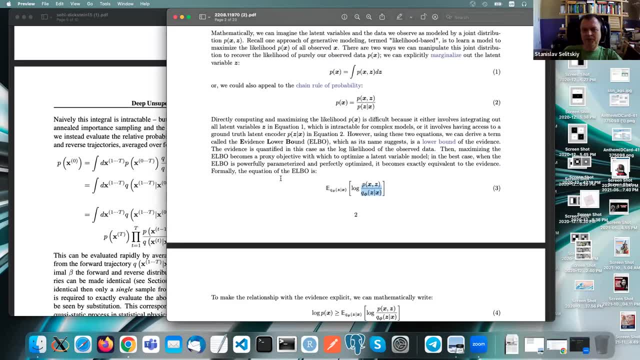 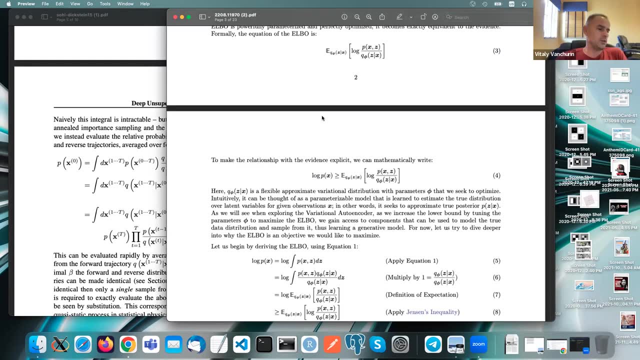 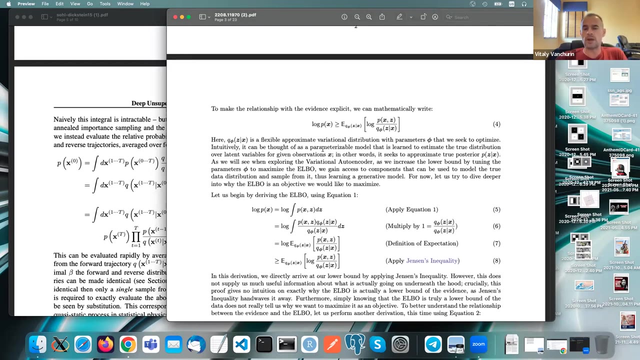 this ideal ones. so they uh. so here is their like derivation. so we have first uh, first equation here. one thing i don't understand: like you have many uh, um non-gaussian distributions and only you know only few parameters. there are many parameters that would describe non-gaussian distributions and then the gaussian distribution would. 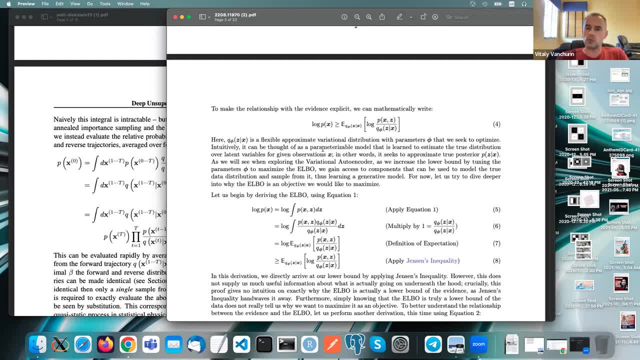 describe only mean and variance, right? and you are saying in your bottleneck you will have gaussian distribution. so obviously you're not going to have enough uh parameters to specify arbitrary distributions in your input. so just one comment, uh, if you don't mind. um so, so i'm not too familiar with this paper, but it seems kind of similar to uh like standard. 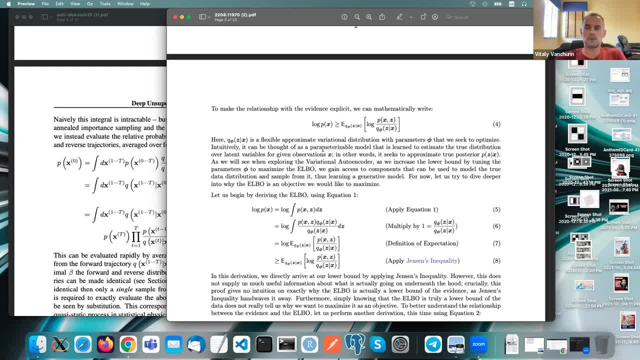 variational auto encoder story. yeah, yeah, yeah, so right, like even this, this stuff with evidence lower bound, i mean i think that's pretty. that's also how the loss function for variational autoencoder is defined. and then variational autoencoder like we have in the bottleneck, we have a gaussian distribution. 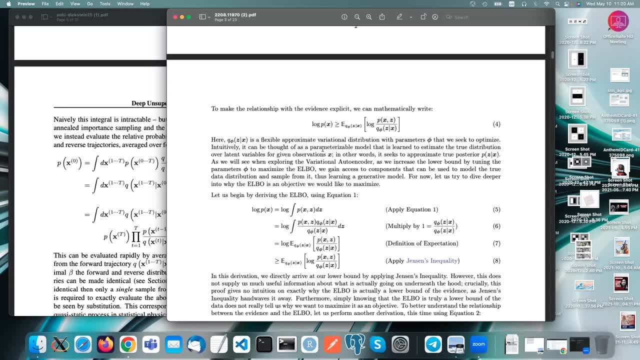 essentially right. so everything is just specified by mean and variance. so mean and variance contains some information, and and then that is decoded through decoder. so is it kind of the same story? here is just like the way encoder works is uh strange. yeah, yeah, so, other than yeah, yeah, so. 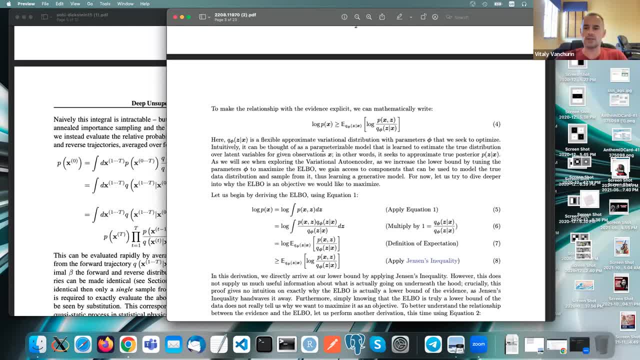 they start. what happened with all the other information? that's my question. right, so if you only keep mean and variance, and there is a lot more, uh, where is it all stored? so we have this like multiple layers and all this information is stored there. so basically no, no, but but. 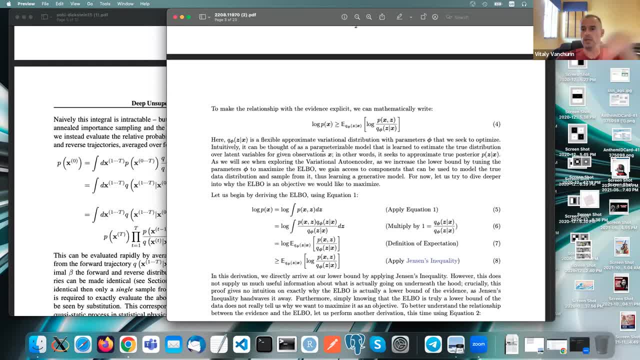 you even some data from the bottleneck, right. so any, any data from this distribution on the reverse path presumably will produce an actual image, right. that has this is very non-gaussian, uh yeah, so so it will have a lot more complexity than than just the gaussian distribution. so i 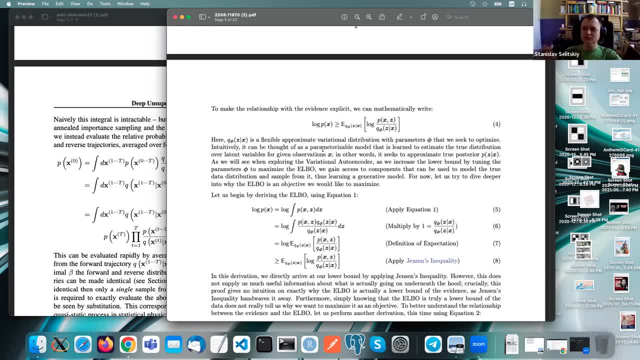 think i'm missing something. yes, yeah, like, basically, to store all this complexity we need multiple layers. so, uh, like, basically, in no, no, to decode you need multiple layers and then code too. so, basically, but to store it it is uh, yeah. so, uh, maybe maybe it makes sense because you're starting in the distribution, even if it is a trivial. 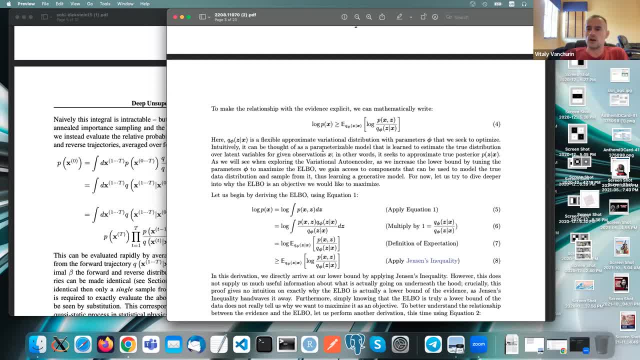 distribution like flat, somehow it records, uh, all of the features. i don't know. maybe it does make sense. yeah, i'll take it back. yeah, and this is even if you just look at mean of, uh, gaussian distributions. right, that contains some information, right? so you need multiple layers and then you need 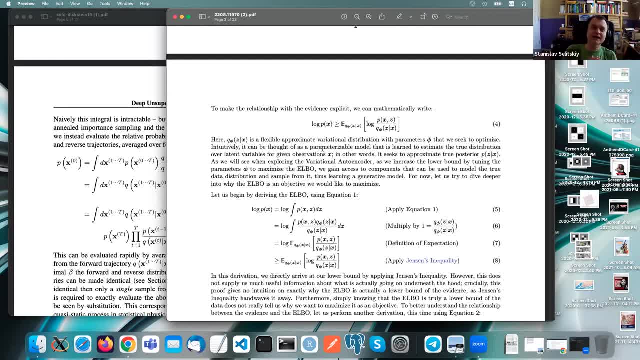 so you need multiple layers, and then you need multiple layers, and then you need multiple layers, Yes, and then distribution. and if we have, like many of these distributions, and they are all connected, like the dependent on each other, so we store this information on each step. 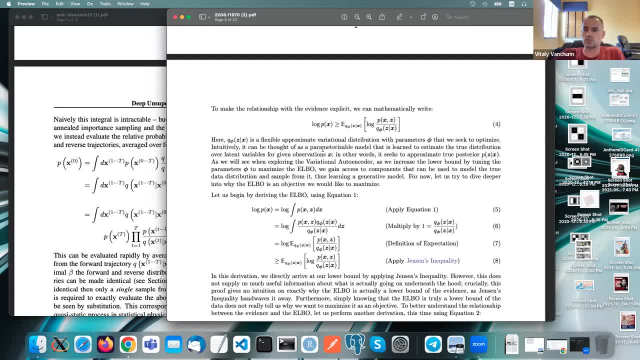 Okay, so maybe the way to think about. let's say, you have complicated function which is now, of course you can like, converted to the Gaussian by squeezing certain areas and stretching certain areas, And so very complicated shape of the distribution would still be, you know, possible to just describe by Gaussian, given that you can do all the stretches and squeezes. 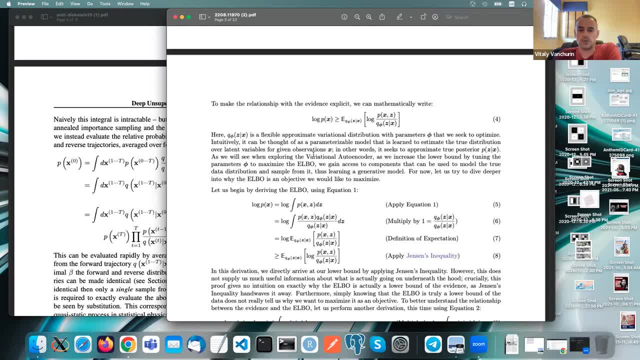 And then basically, that distribution will be in the one to one map, with the more complicated one, And that one to one map is what this encoder and decoders are. Yeah, so basically, if we're talking about this, auto generative models- 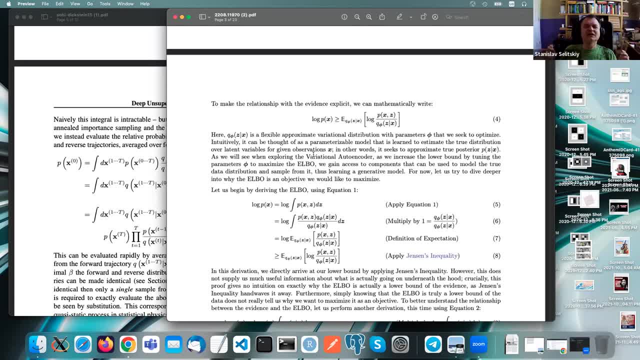 Like. what we want to do Is to like not just models, but like generally unsupervised, like learning. we want to use prior information, some elements of this information to train this model, like to generalize, like to learn. other information like we don't have. 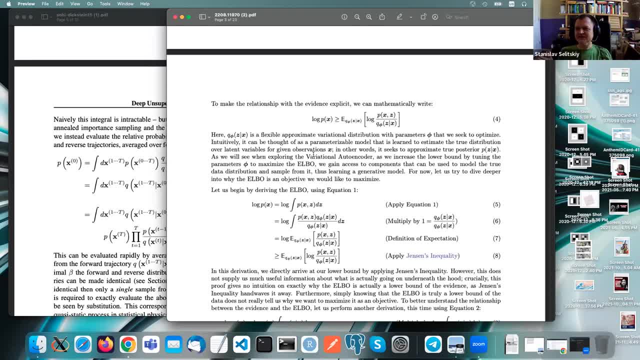 And here we some kind of like looking like keys under the like streetlight. So we say, if we Like corrupt our initial data like long enough, by small steps we will go to like pure chaos, Like to like Gaussian. And that is our prior information we extract from the input data. 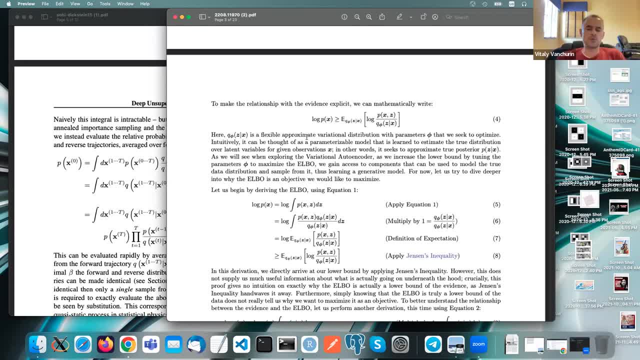 But No, I don't think it's a pure chaos, It's just it looks like Yeah, yeah, yeah, yeah, yeah. When you look at the probability distribution is chaos, But actually every given state Of you know Z. 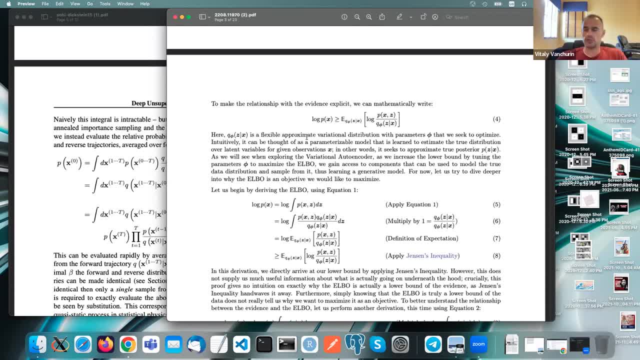 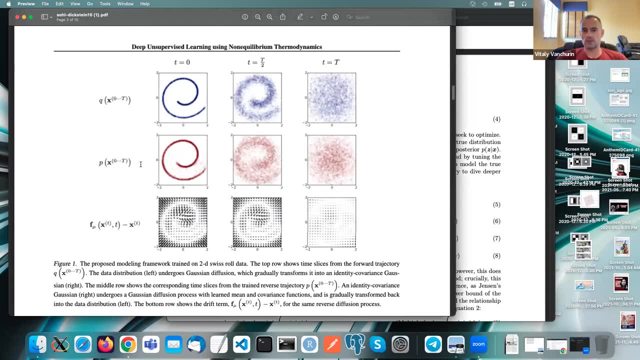 They are respond to some very not chaotically looking Image, And so it is just: you've taken a complicated probability distribution and converted into the very simple one, For whatever reasons, And then and then all of the information is, from that point on is just in the weights and biases of the encoder. 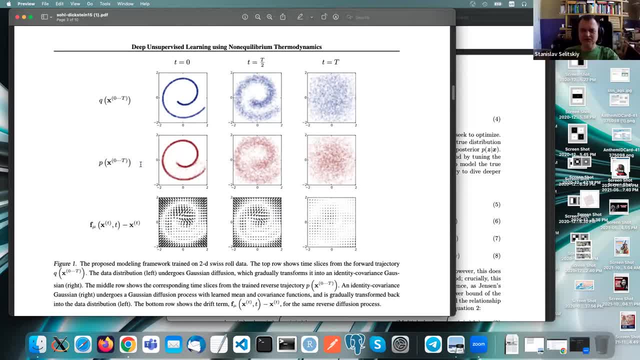 Decoding In the regional like paper they have like really nice. Yeah, Like this is is not like pure chaos, This is like final Distribution, How they this like Swiss roll Encoded into like Gaussian, So it's. 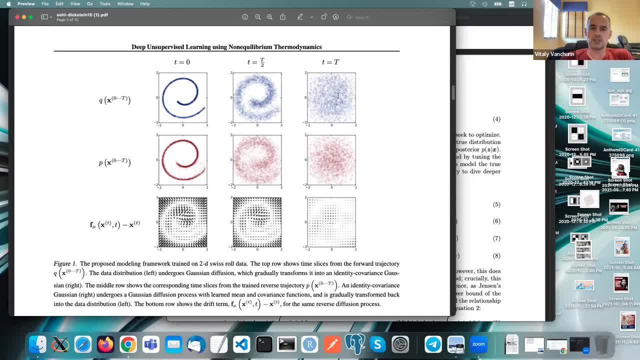 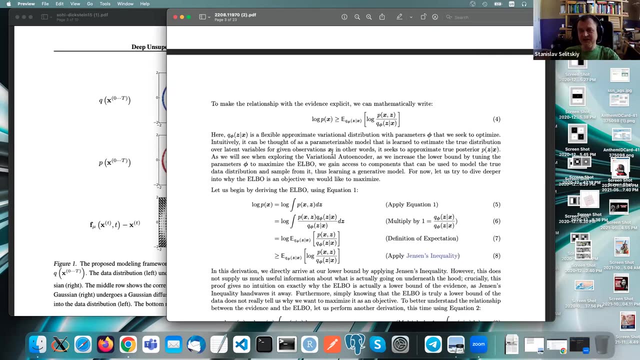 Right, But, but. but the information that is Gaussian is actually this wiggly line, For the line is is exactly in those weights of the output and quarter Decoder. Yeah, And like in general settings, This is exactly as. 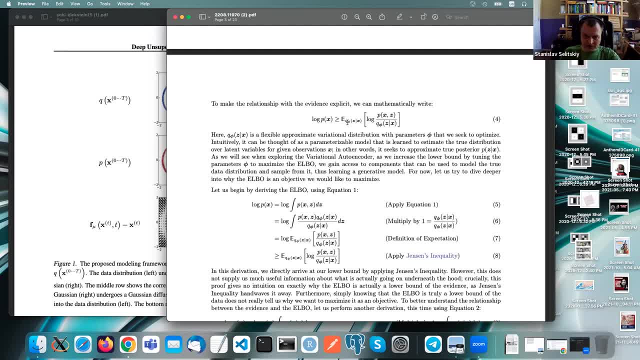 Like generic variation, Encoder This, Like there A fee which is like vector of all possible parameters. So we're not talking about diffusion yet- Like it could be really a large model with millions of billions parameters And we can use. 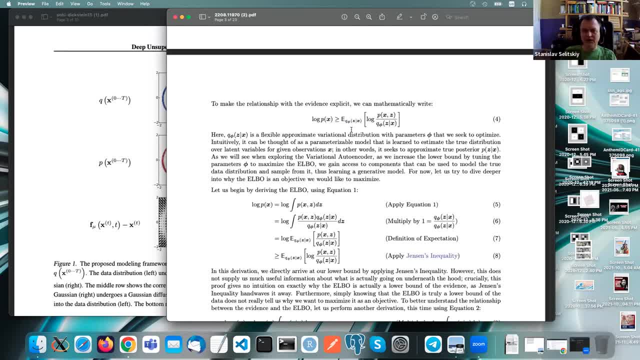 Thunder Network And store all this information here. So when you say diffusion, it's you really mean that kernel, What you called Conditional probability, right, You just mean that this kernel has a certain structure to it. Right, Diffusion like structure, but in general it is a mark of chain. 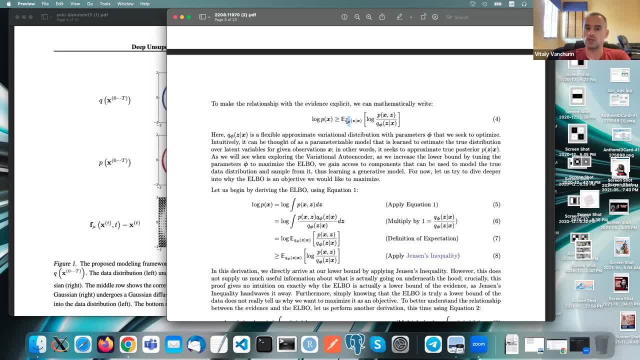 That takes you from there To a Z. What about the backwards path? Now it's not longer diffusion, It should be some kind of anti-diffusion. Yeah, this is like, exactly Like, Like kind of Anti-diffusion. 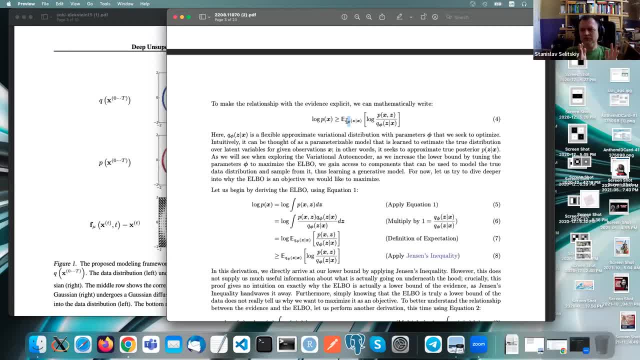 So we basically Use Previews. So our Like diffusion step And we try to find inverse for anti-diffusion And like we Like, because we have this really small steps, We can linearize and have some kind of. 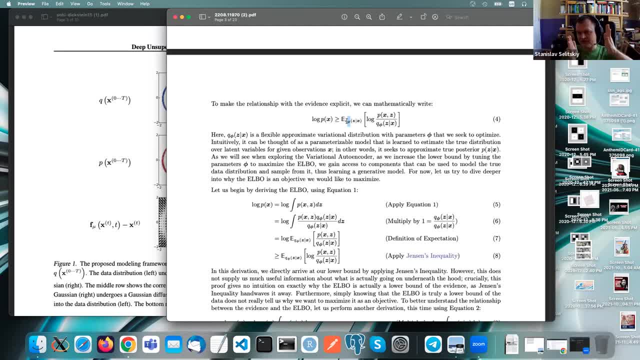 Continuity of Direct transformation on the Like, a conscious step and Same step Of Decoding some kind of. But hold on, Encoder and decoder are trained separately. It's not that one is the inverse of the other. I think they could be. 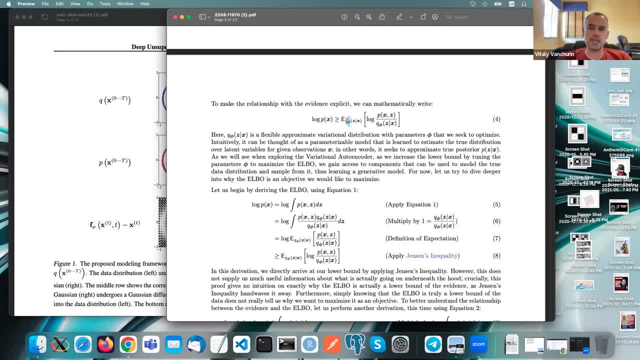 So they have. There is an ask If they would be the same. We do know that, Like anti-diffusion, equations are very unstable, So you cannot just write anti-diffusion information, start solving it. Then the high frequency modes will just blow up. 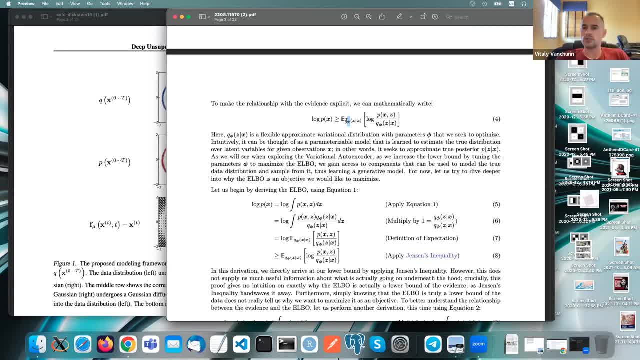 And then like small numerical instabilities will blow up. So that's not going to work. Just just reversing the diffusion equation. But maybe if you are training for those parameters Then this kind of Handles medically They have different optimization parameters for. 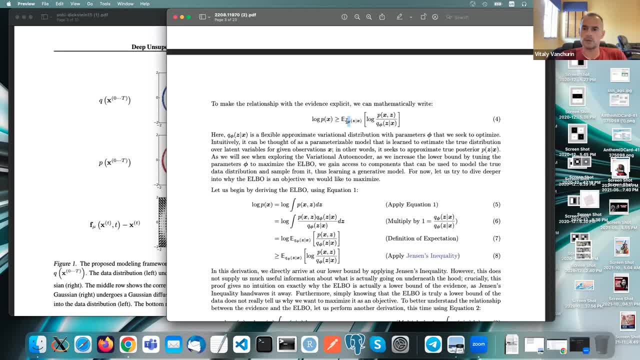 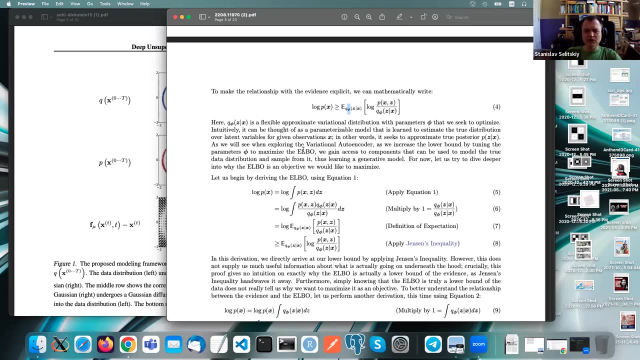 Those two passes About how they do this. I'm not sure. Maybe, Yeah, Like, maybe they They train coder freeze, Like this is A little bit, But Like we stuck on on like this step, So Like here, we just like going. 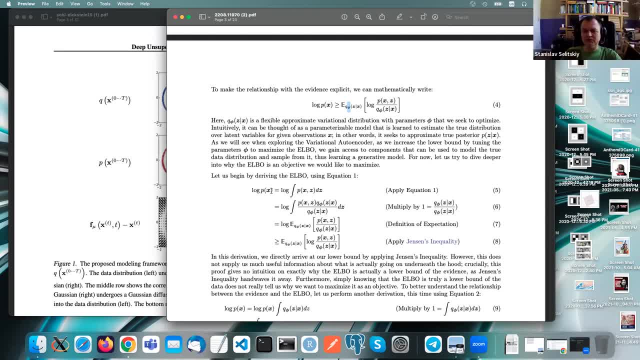 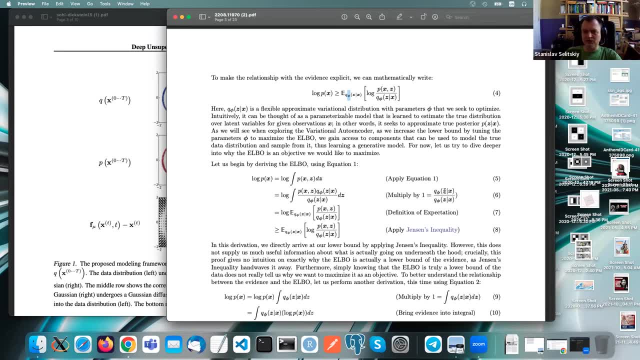 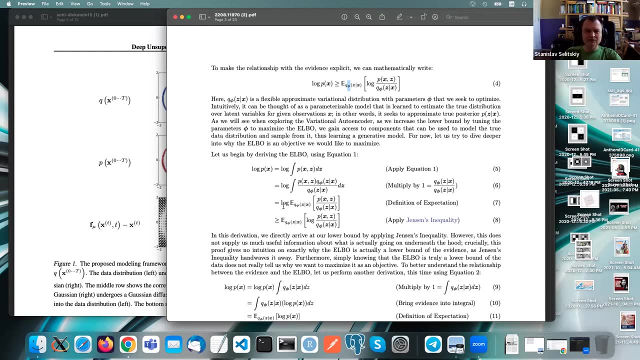 Like pretty trivial things. So like from our regional Marginalization equation We take like logs from both sides. We multiply by one, Like this division. Then we Like say like this is Like basically definition of expectation. So this is: 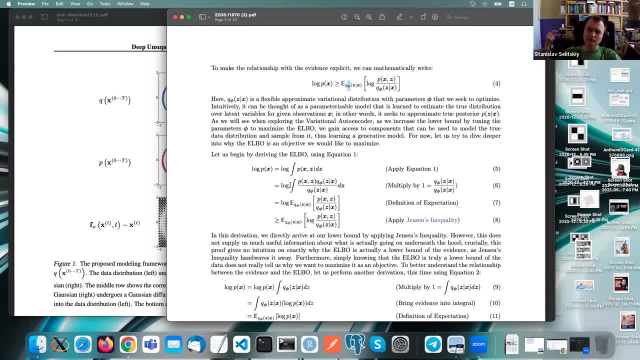 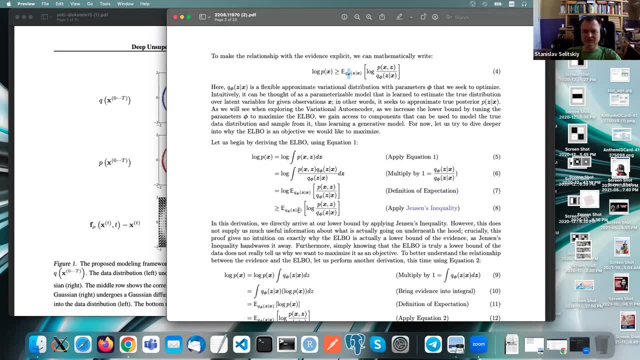 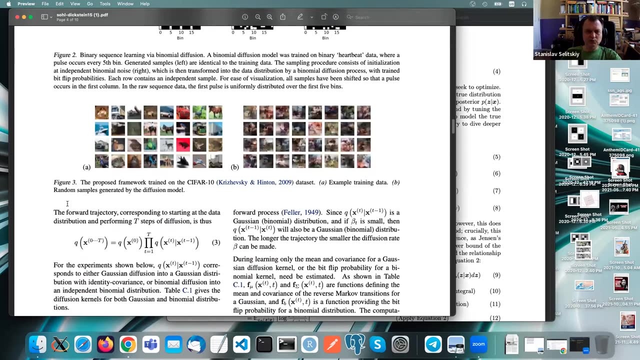 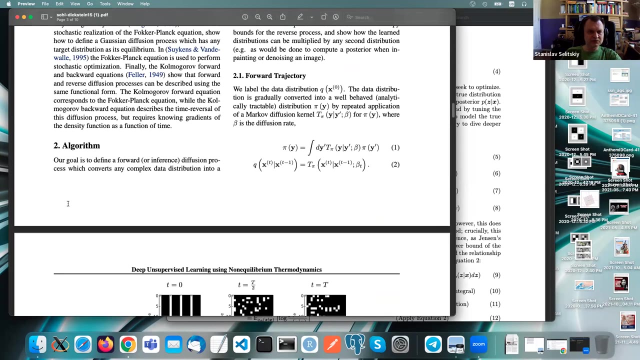 Some of the Like value multiplied by Probability. And then we have this Like Like Janssen- inequality. In this paper They refer to Like, more Like physically, like physics, Like use, Like another name, But But basically this inequalities. 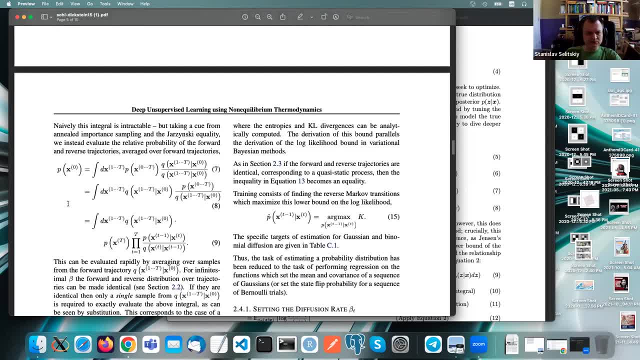 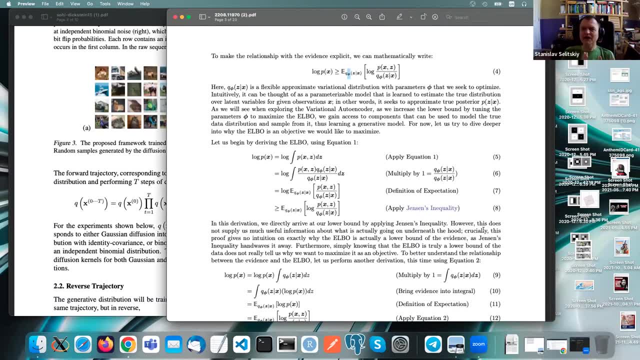 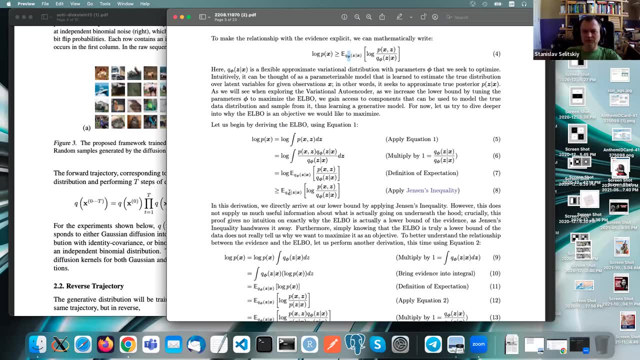 Are related, Become Like to the same one. Like, which is Like, basically says That function from Like expected value is greater than expected value of the function. And so we come to this term And we say, Instead of Like, optimizing, maximizing. 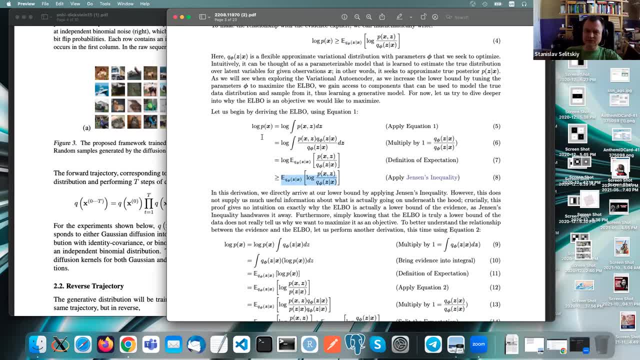 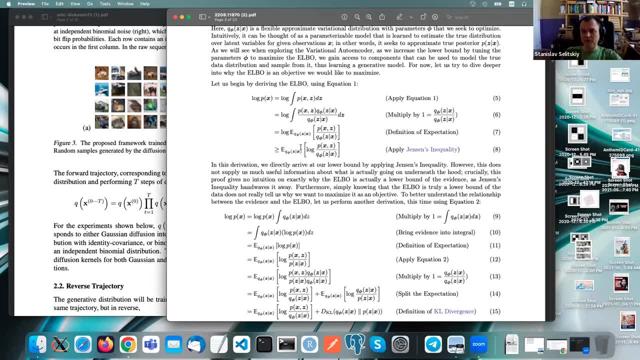 Our Like marginal, X, Like distribution, We want to Like to maximize, Like this Lower bound. And Here They Like another approach, They do Like, basically they say Same. They start with: Like this equation: 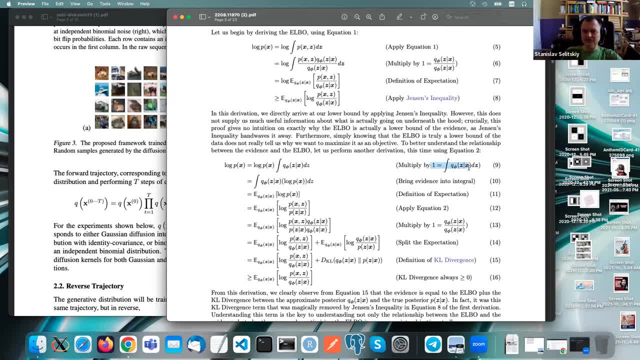 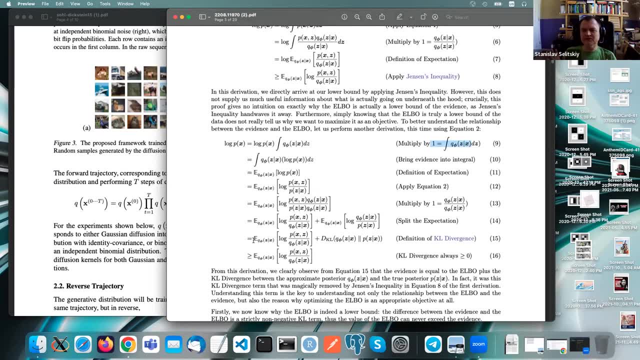 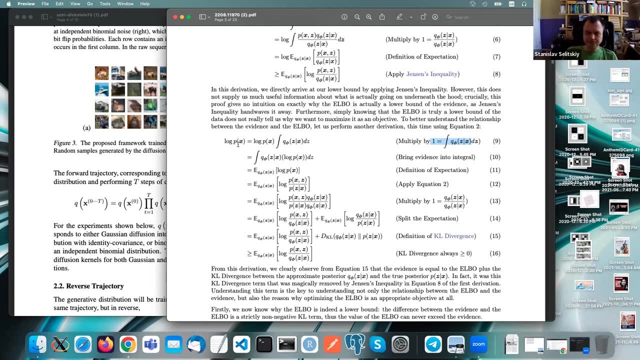 Again, They multiply by log Like and go there And Here They say We see Here Some kind of intuition. So We have This. Look Like. This Log Like distribution Consist of: 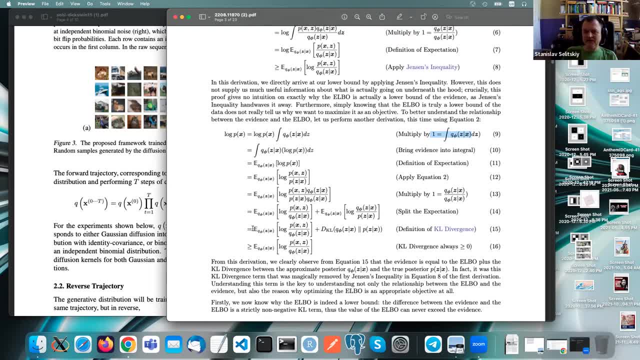 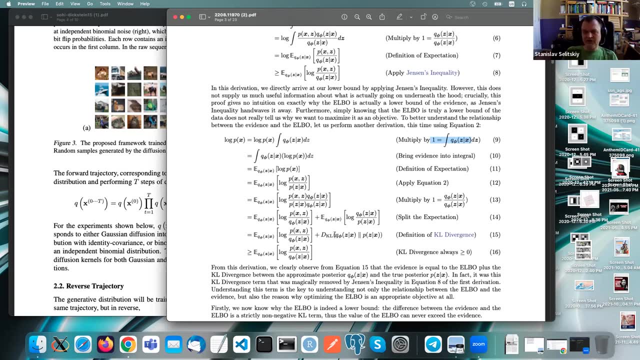 Again Like this Lower bound Plus Like divergence Between Two distributions. So We have One Is basically Our Like final one And Like Like theoretical one. But we want to Get to So 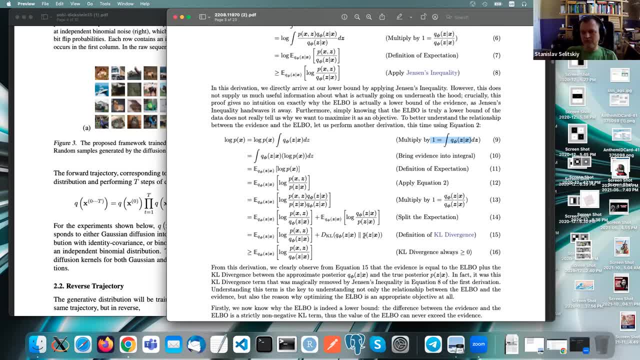 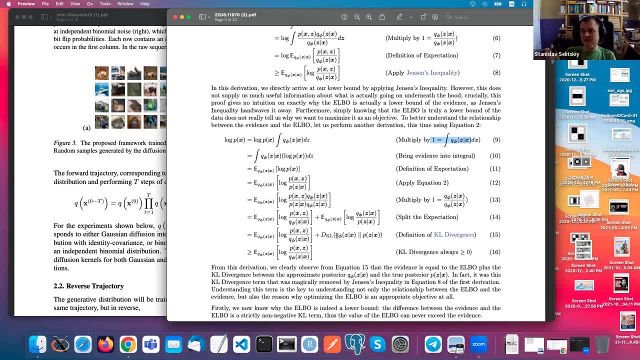 Basically This is Like Gaussian And Here Is Like Our Learn Distribution On The Final Step. So Basically, Yes, So We want to Minimize This Term, But 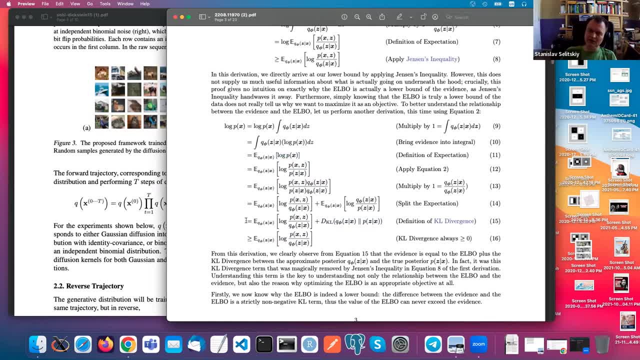 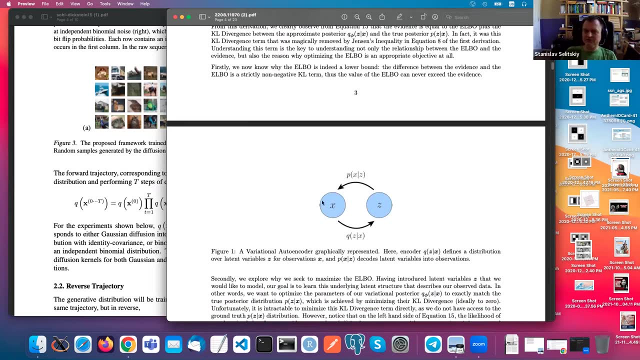 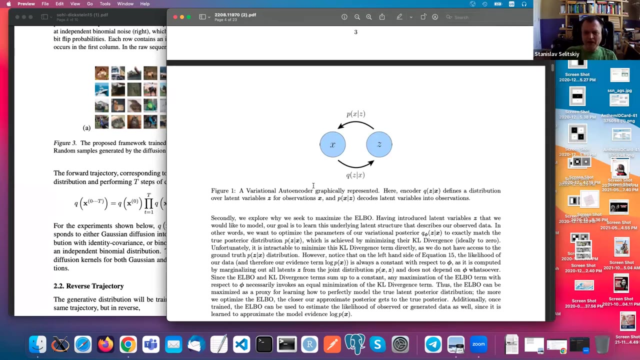 That Mean We Want To Maximize This, And Then They Like Basically Training, And So We Have Like One Step Variation, Encoder As They Like. 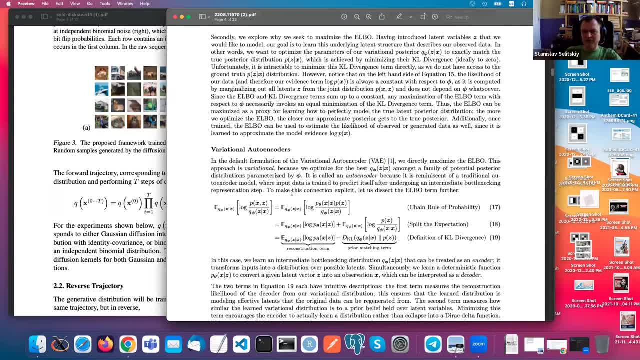 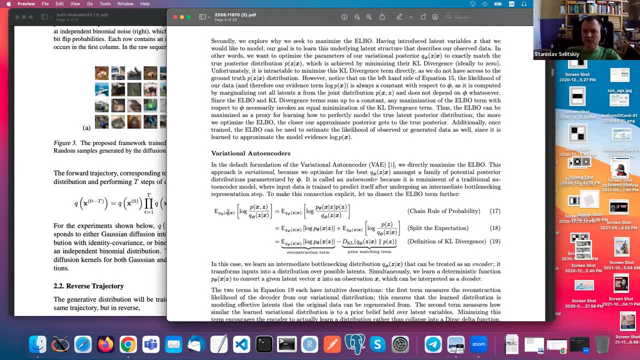 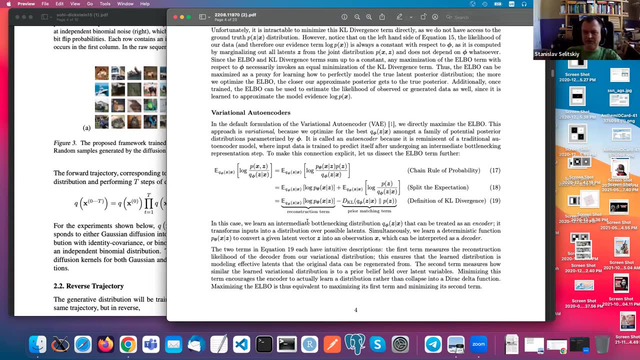 Show Here. So This Is Original Encoder, This Is Bottleneck, This Is Like Back Reconstruction. Yes, So We Have Two Like Again Like Two Terms. 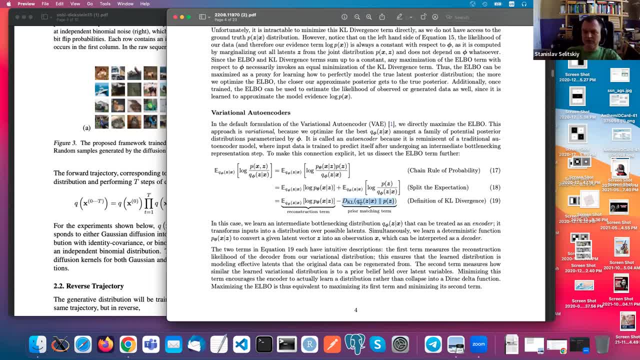 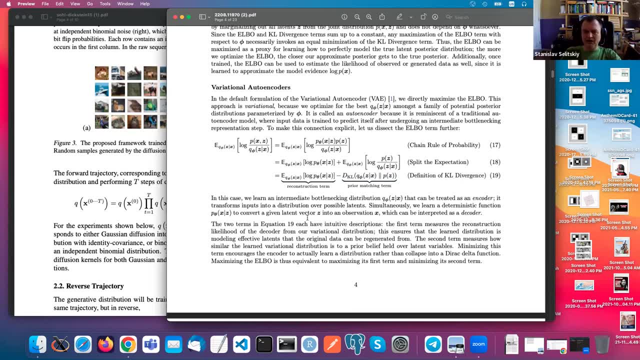 One Is Divergence Between Ideal Gaussian And What We Learn, And They Train To Have It Close To Zero. So These Two Are Like Basically. 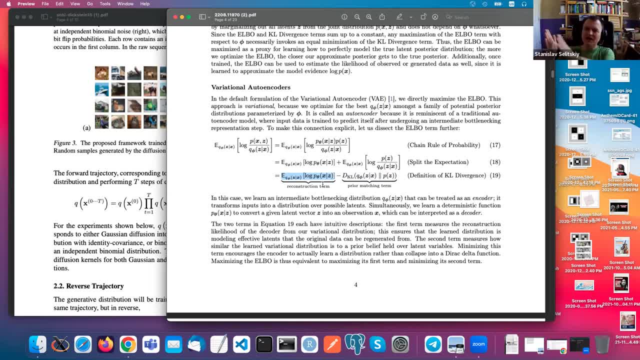 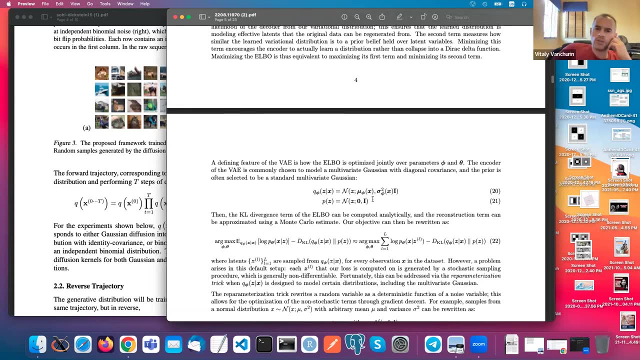 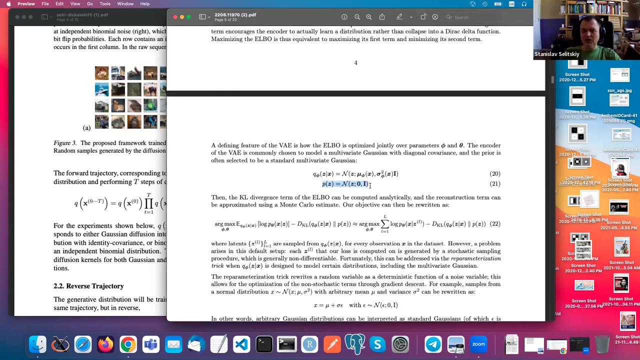 Trained Our Encoder To Represent Gaussian, And Then And Then We Want To Train Our Second Step, Our Decoder, To Original One. So We Want: 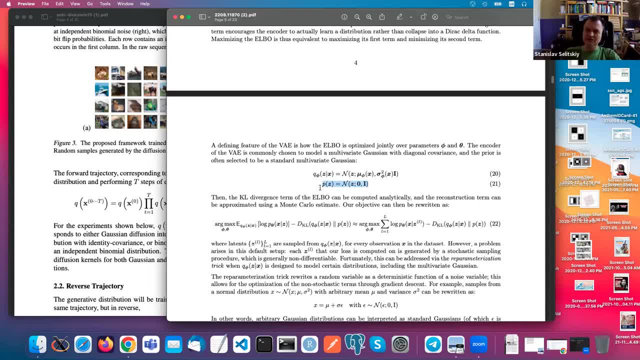 To Train Our Encoder, Like Typical Approach. Yes, In Bottleneck We Have, Like, Basically Normal Distribution And We Want To Like, Make Our Like, Learn. 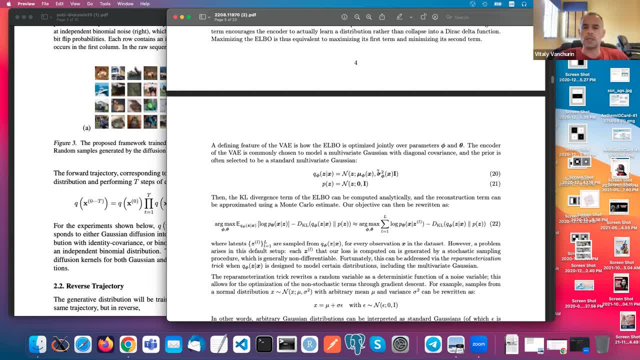 Distribution Like Based On, Like Learn In The Bottleneck. What Does Make It Variational? What? What Is Really Being Varied Here? That's What I'm. 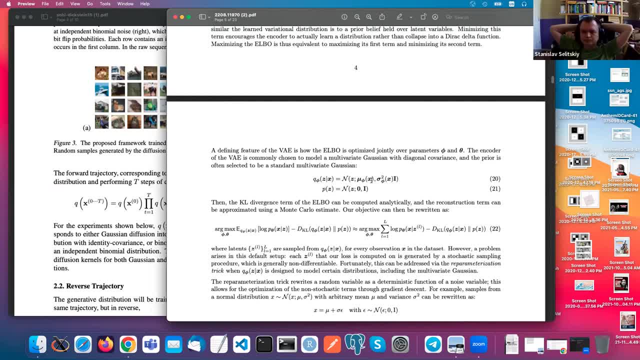 I'm Not Sure Understanding What Is No, Like I Mean There Usually: Yeah. So Basically, We Want Like, We Want This, Like You, So This. 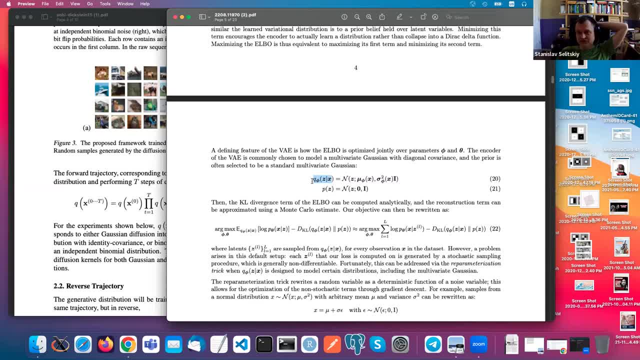 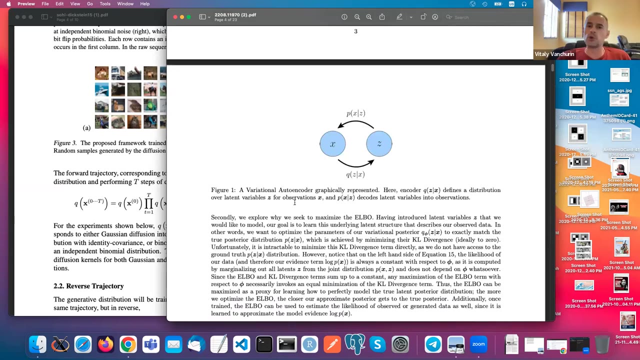 Is Some Kind Of Little Bit Like- Not Very Strong On This Part, But This Idea That The Learned One, The One You Learned, Can Be. 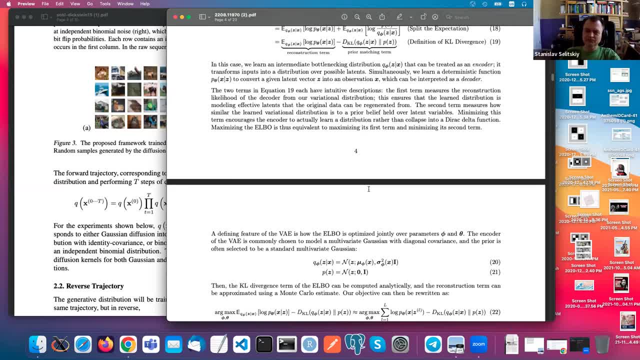 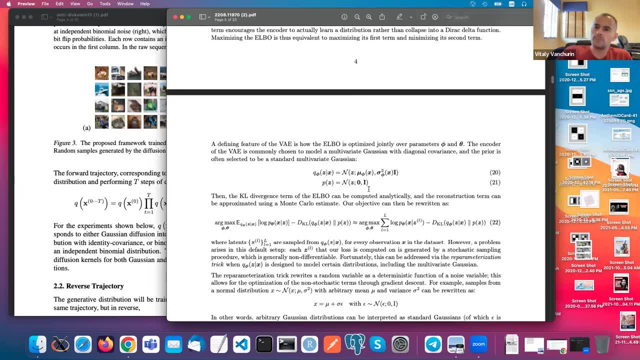 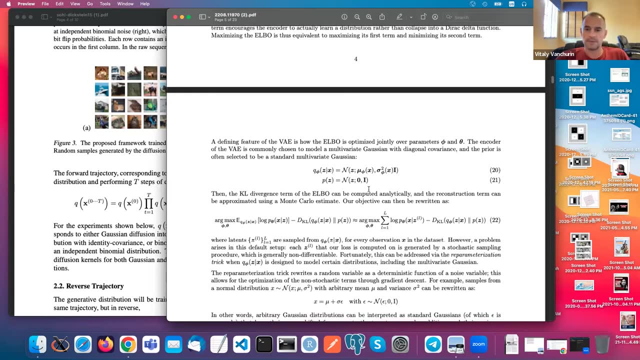 Anything At All. Yeah, Yeah, Like I Mean. Yeah, So They're Like Bookkeeping Of That Distribution In The Bottleneck. Yes, So You Think You? 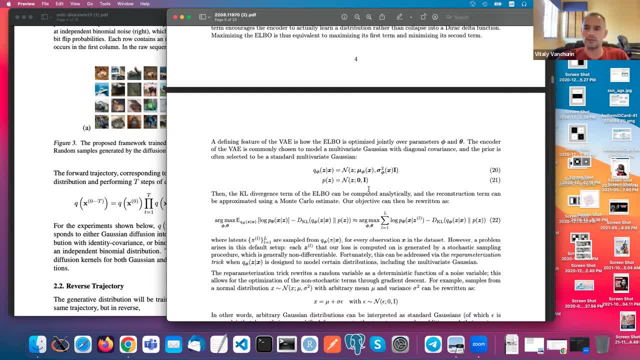 Think Variational, Like The Same As Gaussian. At This Point I Think Yes, If Like, Because Basically It's True That If You Use Some Variational, 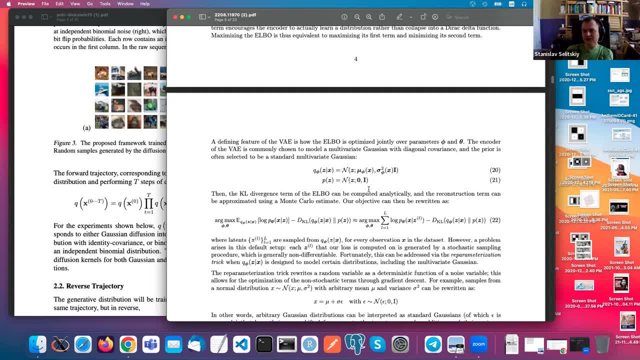 The Way We Want To Constrain To Our Bottleneck. Let's Say Like Exactly. Let's Say Bottleneck Was Just A Flat Distribution. Let's Say: 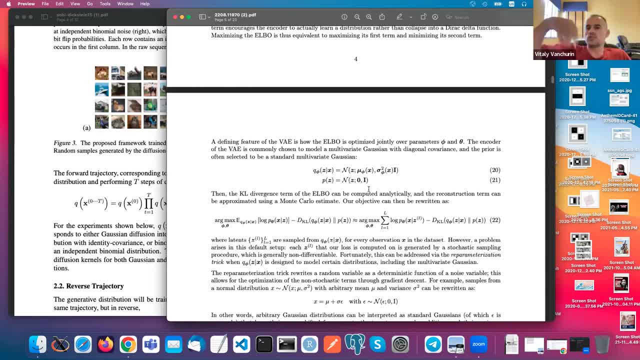 Flat Between They Know Zero And Force The Condition Such That This Okay Like Because We Might Not Want To Enforce Any Distribution, For Example. 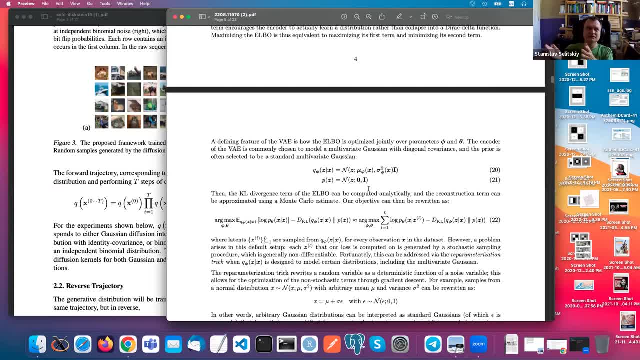 We Just Compress This Bottleneck To Like Minimal Number Of Distribution. So We See Why It Would Be A Good Idea For Them, For The. 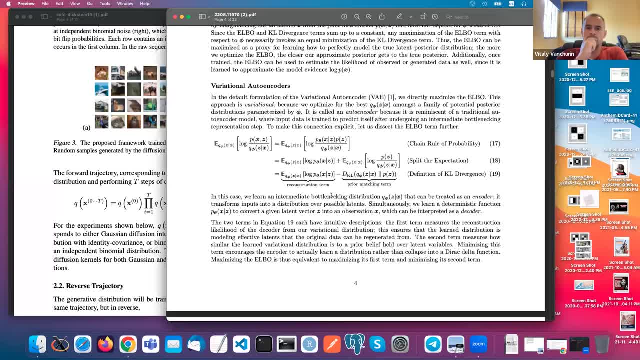 Bottleneck. But Yeah, I Think Another Reason Why Maybe Called, I Think It Might Or Something Like That. Okay, But Then Maybe What You're Saying 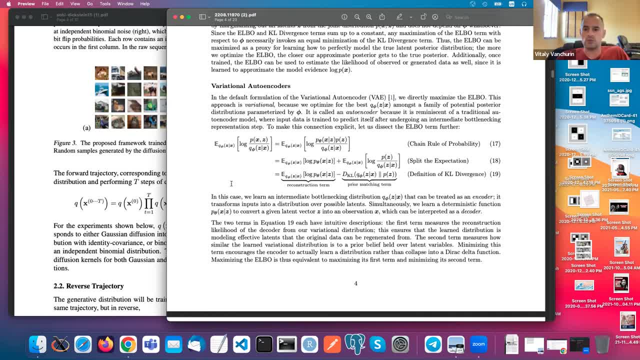 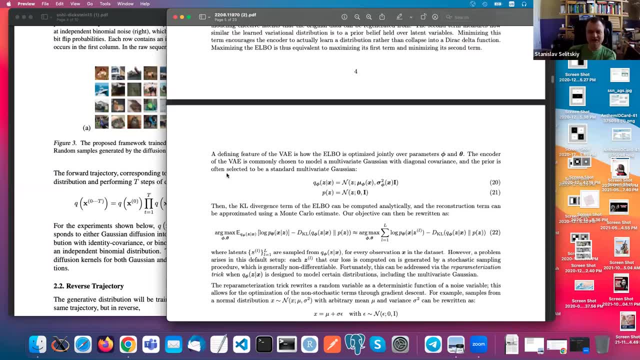 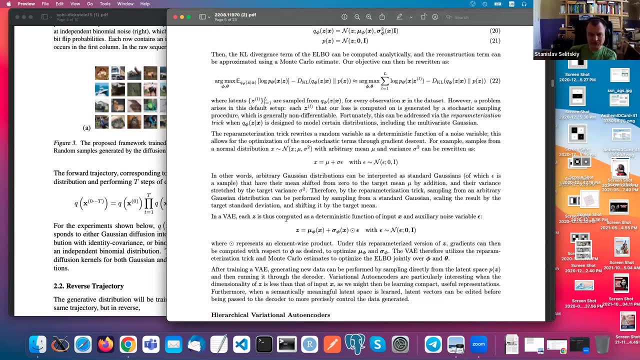 Is That There Is A Constraint Such That When, When The Signal Goes From The Input To Bottleneck, It Is A So Original X We. 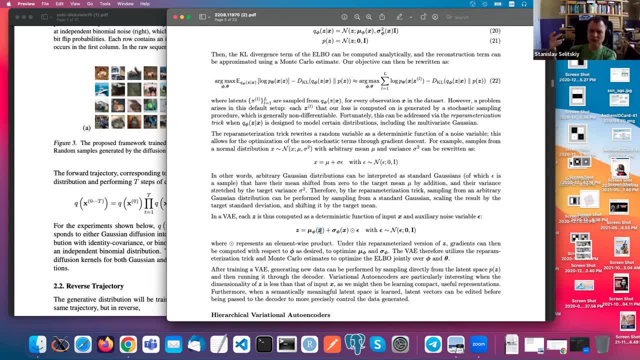 Like. Use It To To Calculate Our Mean On Original Distribution, Then To Calculate Our Like Dispersion Or Variance On Original One, Then We Calculate. 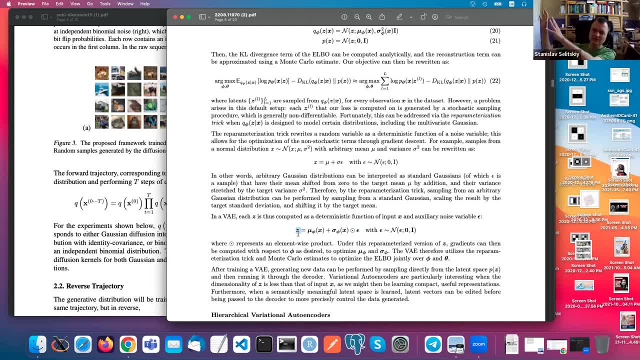 Like Next Like Our Target, Like Next Z, Like Using Original, Like Data. So Instead Of Some Kind Of Like Neural Network, We Just All This. 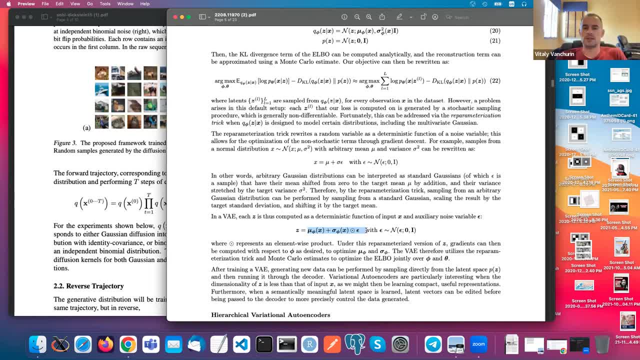 Transformation. We Have Some Distribution To Be Something Yeah, But Like, But For Like, I Think For Variational Encoders Themselves. This Is Not Necessarily. 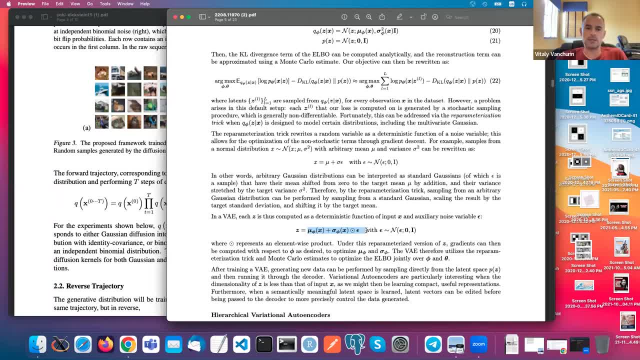 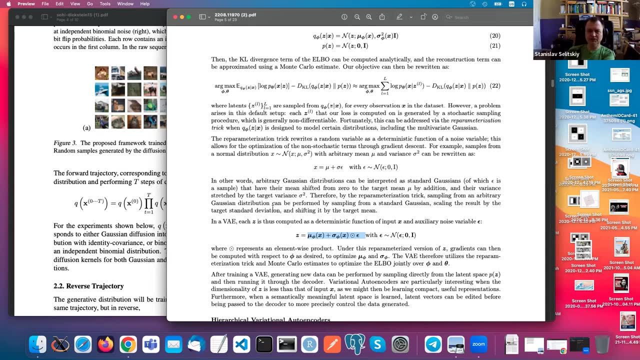 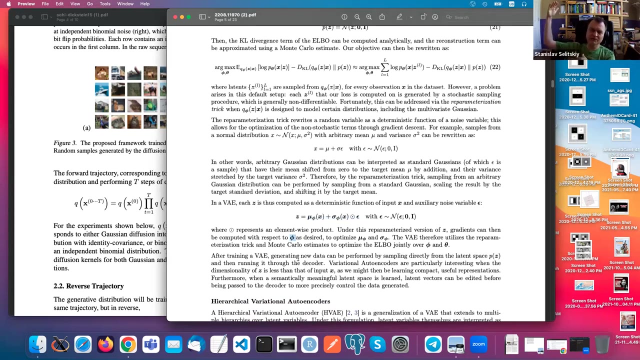 Step, So Like It Could Be Done Right, So You Can Constrain Your Transformation Matrix To Be To Have The Property Of A Stochastic Matrix. 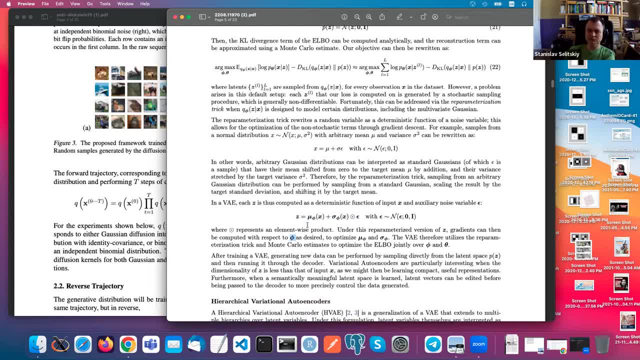 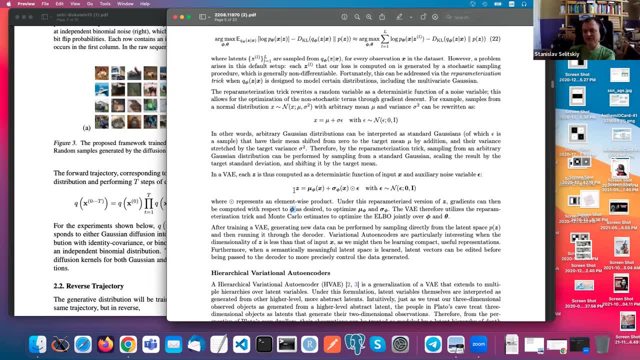 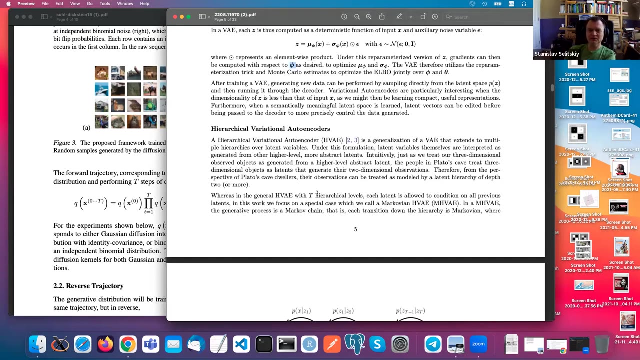 And Then, And So Here, Like, Because We Like Basically Like. This Simplifies Everything For Like For Training Or Like Forward And For Background And 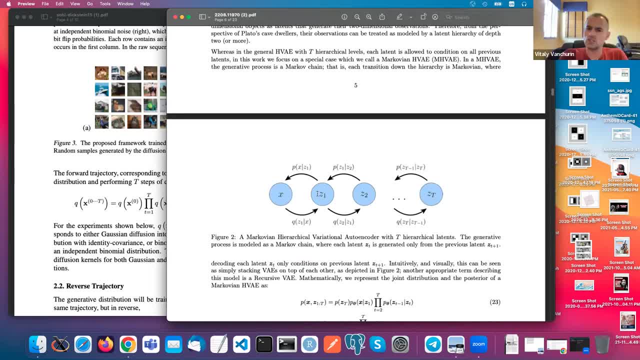 Here They Like Go From Hierarchical, Not Just One Step, But Like Multiple Steps. So We Have Lots Of Yeah. So We, I Remember Yeah. 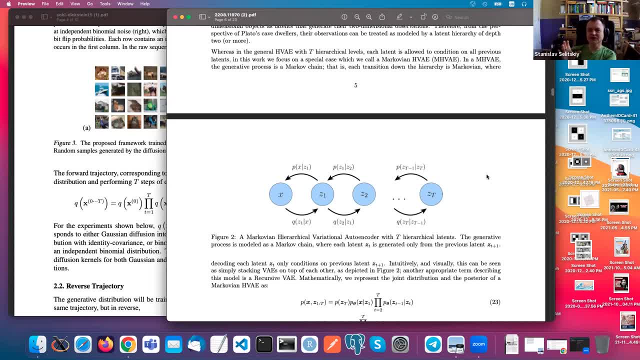 Like I Don't, Like, I Don't Remember Which, Like Paper, Probably In This Paper. They Say They In Terms. Okay, But But That's Fine. 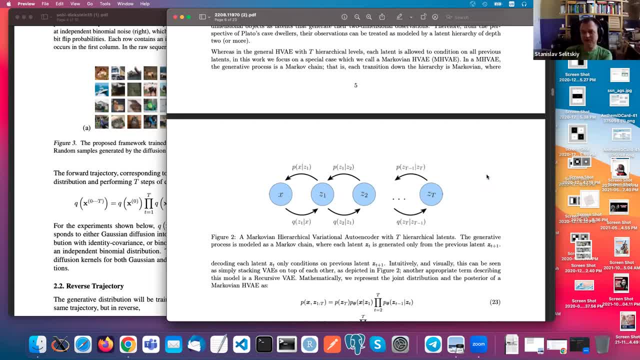 But Then, Then There Is Again: This Mean Is N Dimensional, Yeah. And Then The Covariance Matrix Is Squared. Yep So, Okay, Yep So. 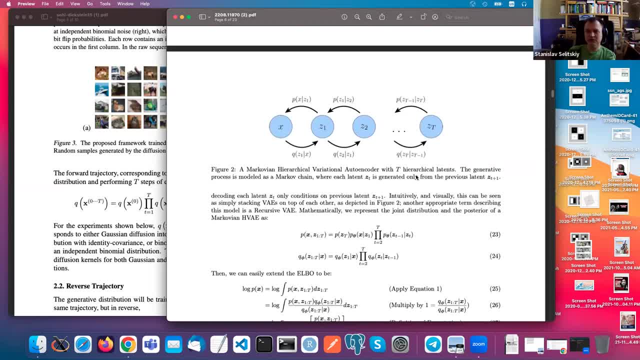 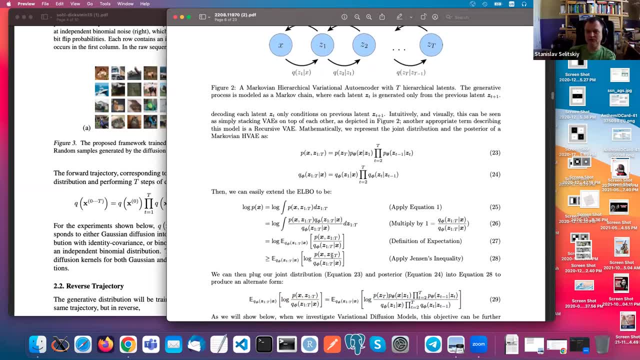 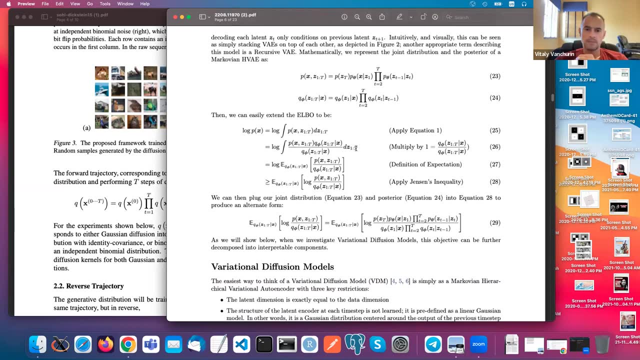 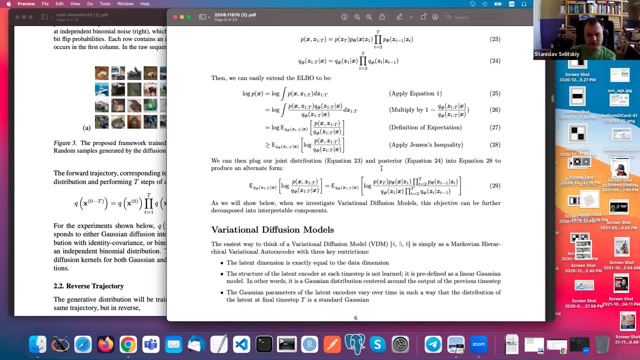 And They Generalize Our Original One Step Out Encoder. It Is Hierarchical Like Multi Step, So We Have This Like Z, From One To T. 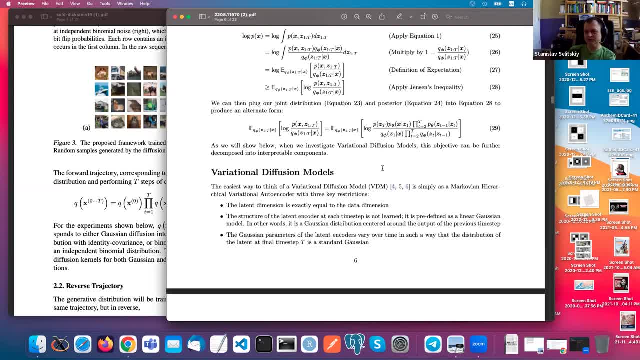 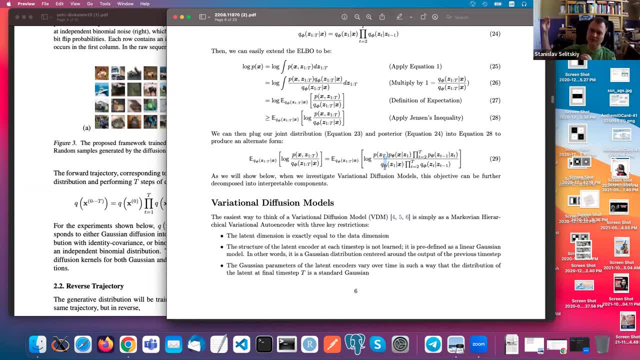 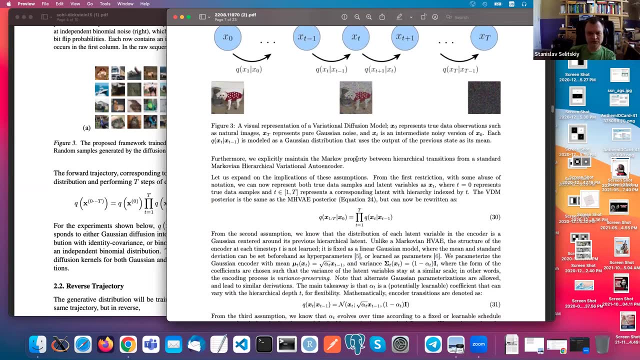 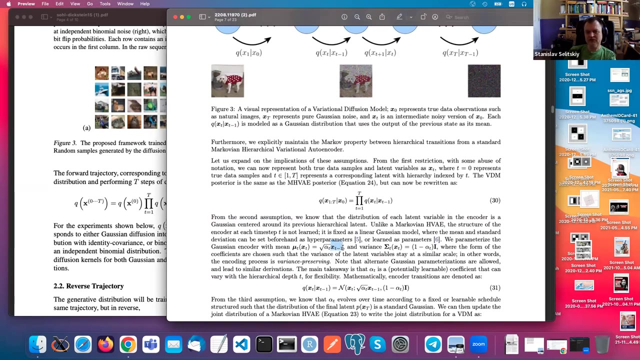 So Basically, Like Like. So Basically, Here We Still Have This, This Term, Like Learnable, Like Parameters Could Be, But Here, Like Again, We Enforce. 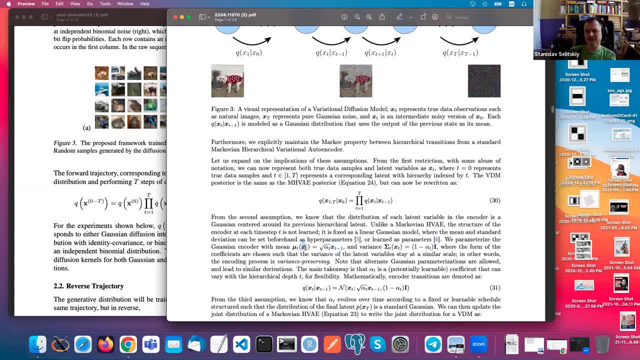 Like, We Enforce, Yeah, So We Enforce Our Like, And This Is Analytically Like Tractable. So This Is Like Analytic Function. We Don't. 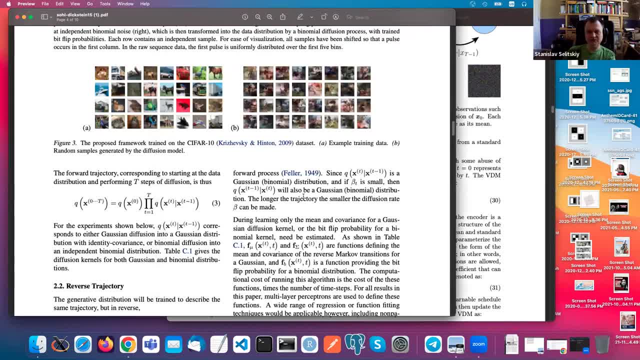 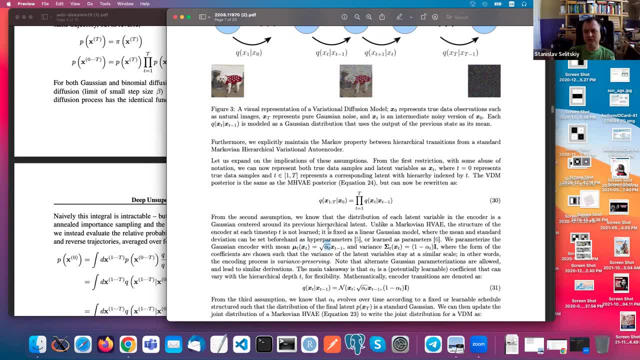 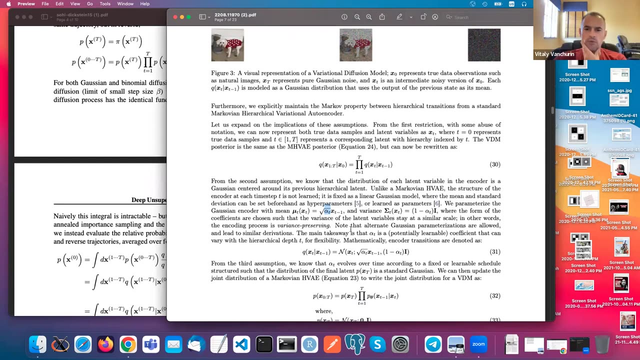 Use Like Generic Function. We Just Use This Like Standard Transformation And And And This As Like Hyper Parameter, Or We Can Like Learn Them So. 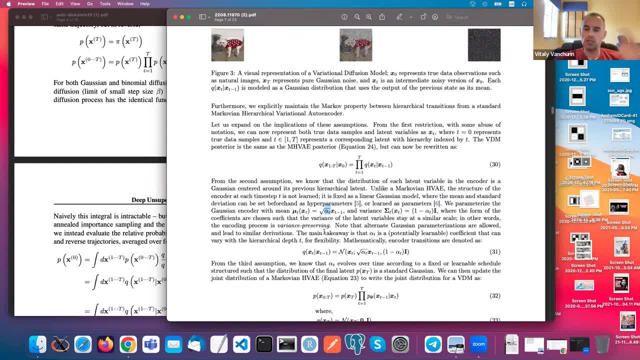 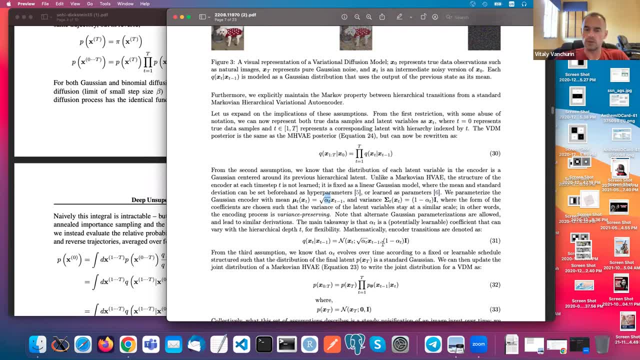 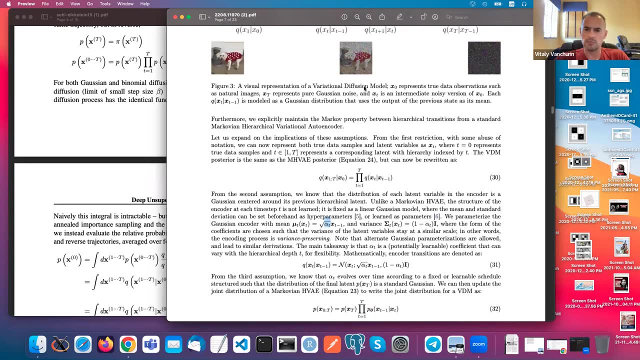 And Then There Is A Covariance Or Variance Matrix, They Call It So. That Means That Each Step, Each Yeah, So They Call It Covariance. 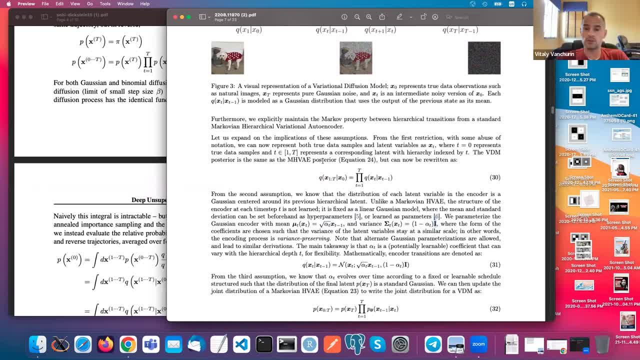 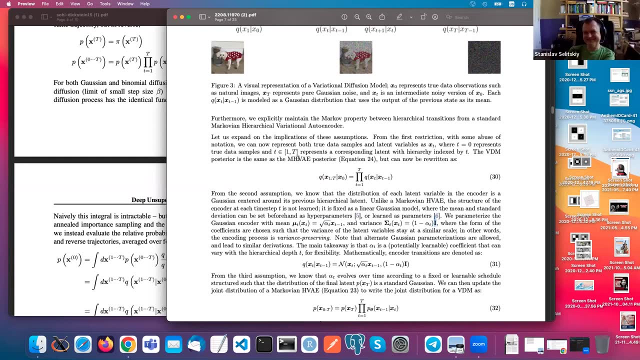 But Basically This Is Like Variance, Because This Is Like: Oh, So They, They Make Each Pixel Diffuse. Yeah, Yeah, Yeah, So They Add Noise. 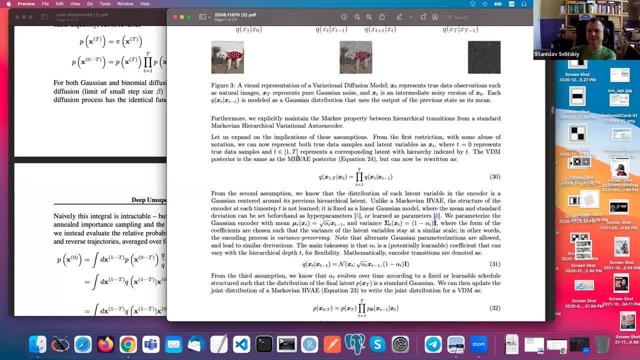 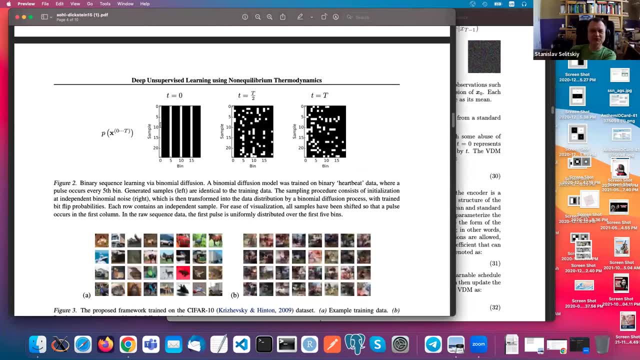 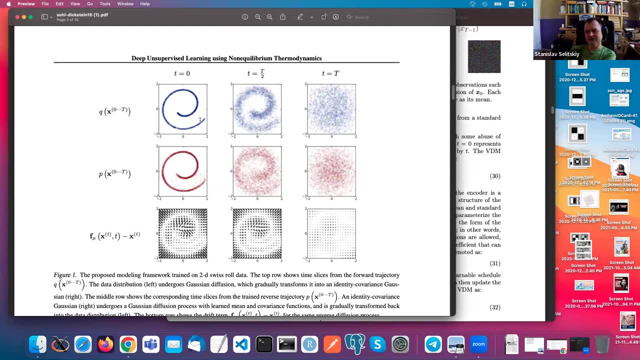 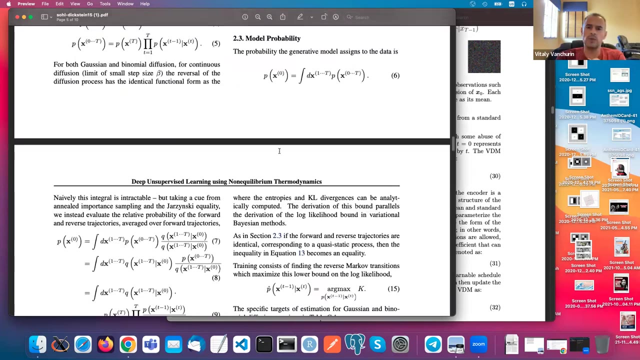 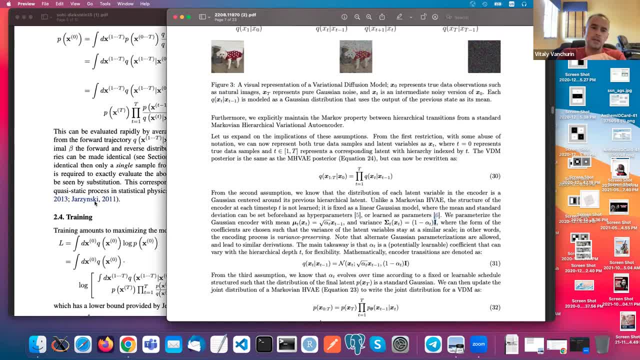 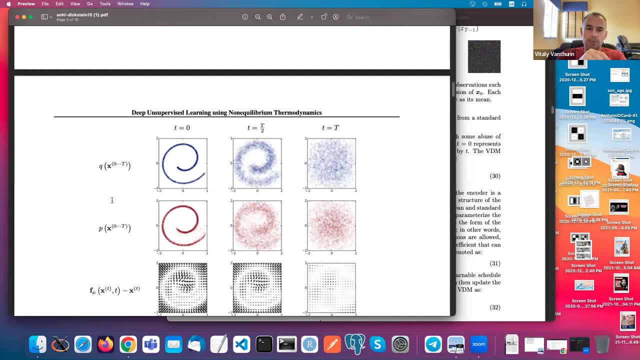 Maybe The Curly Line? Yeah, So If I Would Be Diffusing Each Pixel Separately, Then What Would Happen? The Brightness Of Each Pixel. 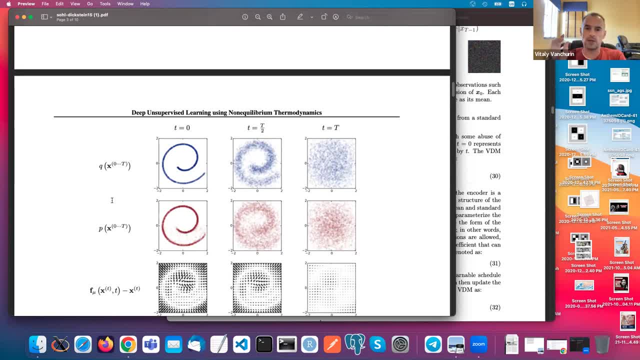 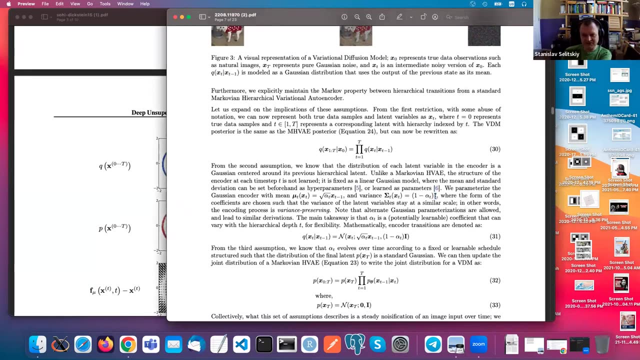 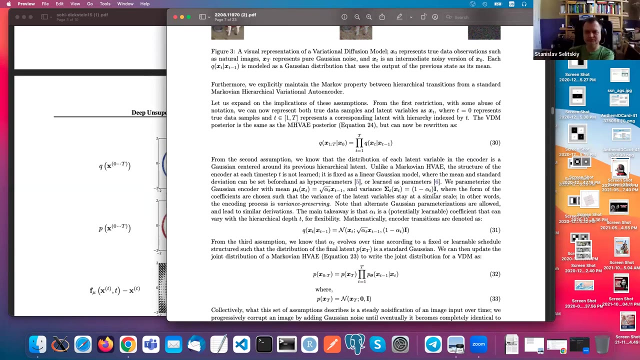 Would Change, But They Would Not Spread Out. You Know, If You're Yeah So You Can Like Diffuse To The Size. Yeah, Because, Like As 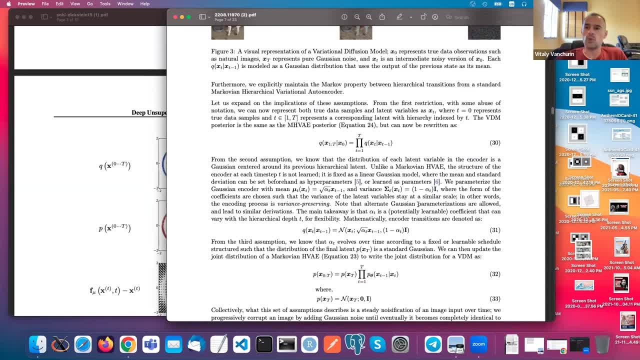 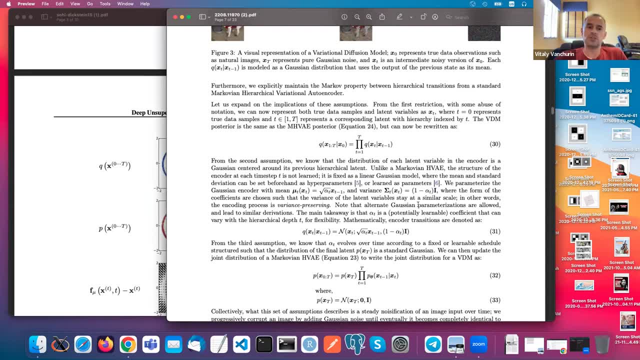 Understand This Is Just Like, But Then That Just Changes The Value. The Whites That Are Closer To Blue Are More Likely To Become Blue. 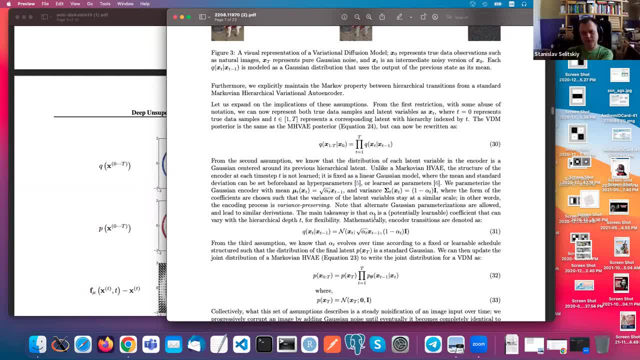 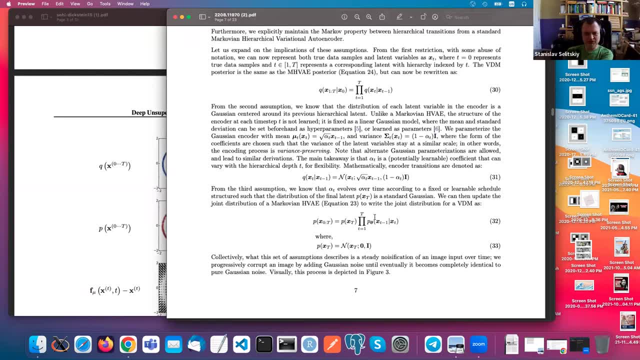 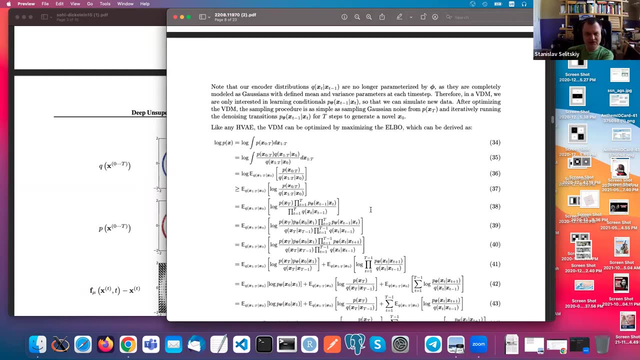 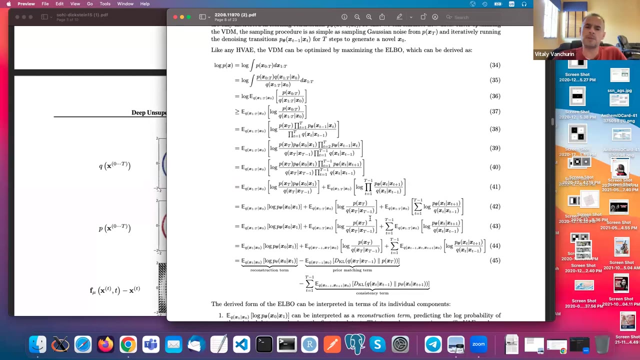 So Yeah, Something Is There Right, Okay, Well, Anyways, There Has To Be Some Kind Of They Trying To Use An Equation For Hierarchical Model. 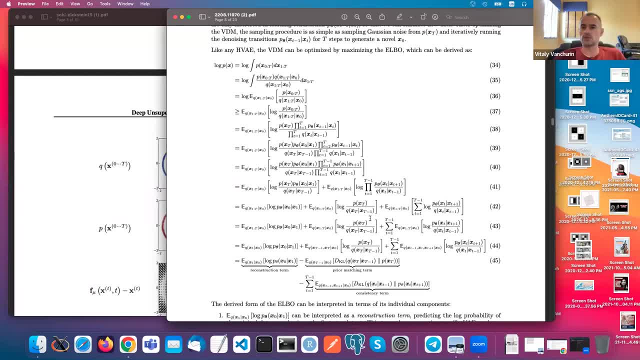 Yeah, But Maybe, Coming Back To My Question, What Is It Good For? I Mean, What Is This Used For? So, Basically, Like Probably They Using 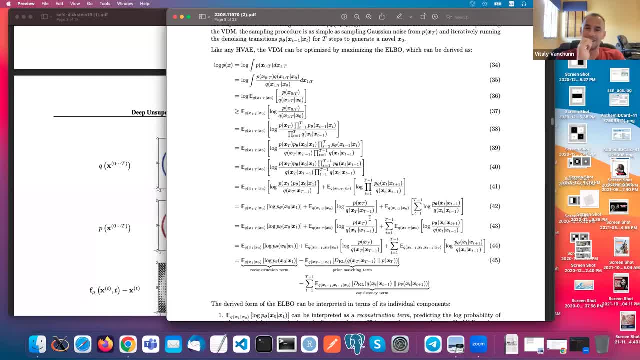 Same Approaches Like: If You Want To Understand Something, You Have To Break Something. So When You So, And Like In Them, So Like They. 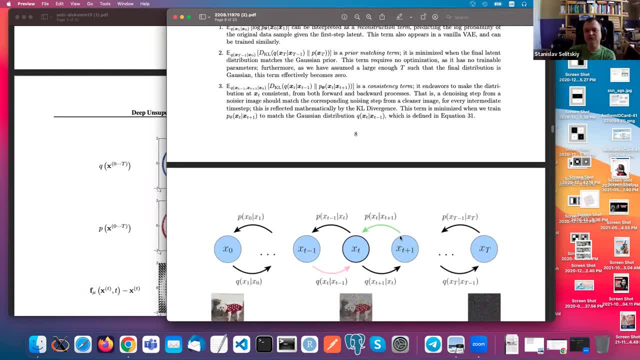 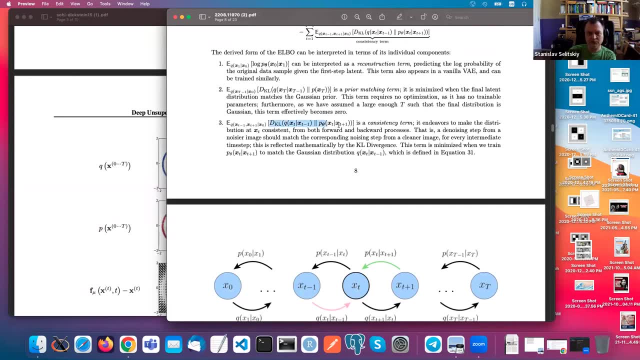 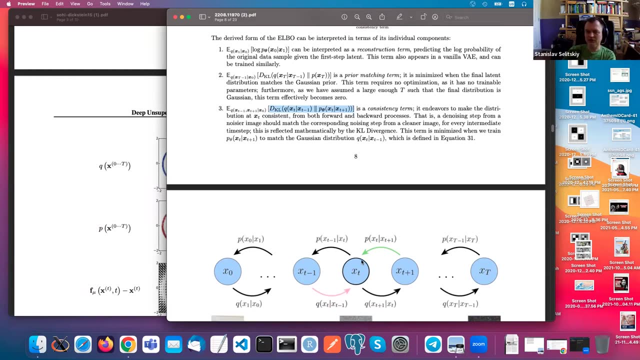 Show It Like Down There: Yes, So They Want Like To Sing. So Basically, They Add In This Divergence: Yes. So What So We Have? 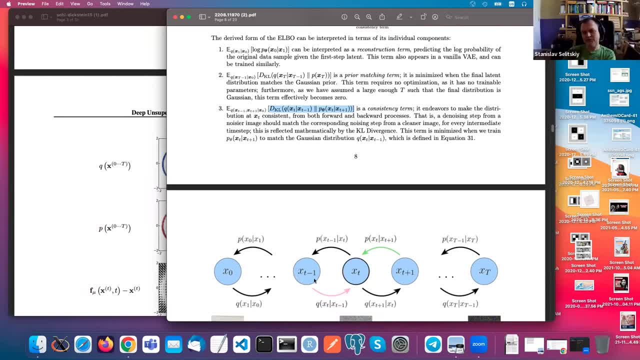 This Like Distraction, Like From The Laptop, And We Like, We Try To Like, Teach This Decoder To Be Inverse, Or This: No, No, I. 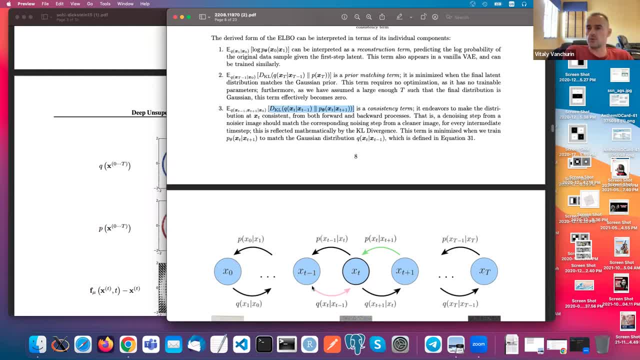 Understand That At The End Of The, So That I Understand. But I Guess My Question Was: What's The Advantage Of Using Actually This Diffusing 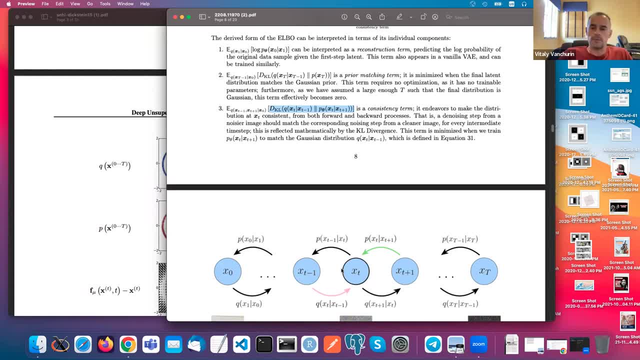 Kernels. Basically, You Have Kernels Which Take You From One To Other Parameters, And So It's Easier To Train Something Like This, And I 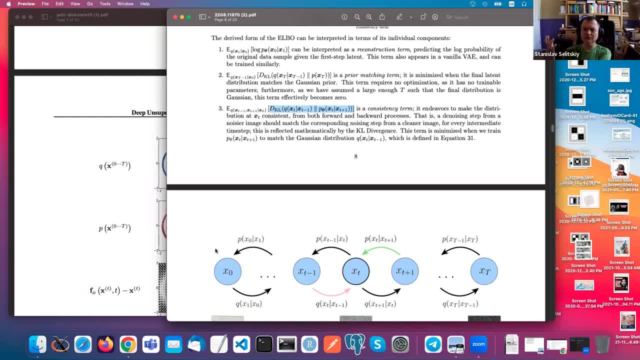 Think They Trying To Do Some Kind Of Linearization, Because If We Have Just One Step, We Have Some Kind Of Linearization And We Have 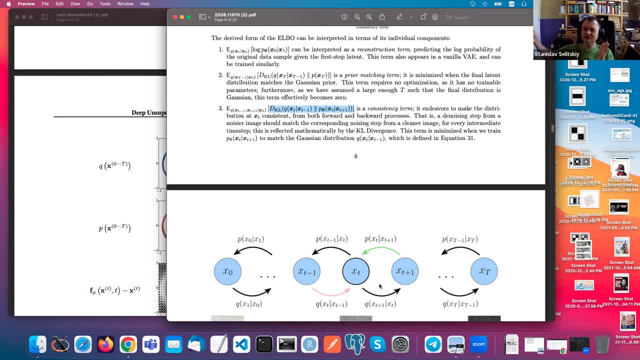 Some Kind Of Like Piecewise, Like Mutation Of The Like Complex Hyperspace With Linearize, Like Fragments. I Think This Is Something That We 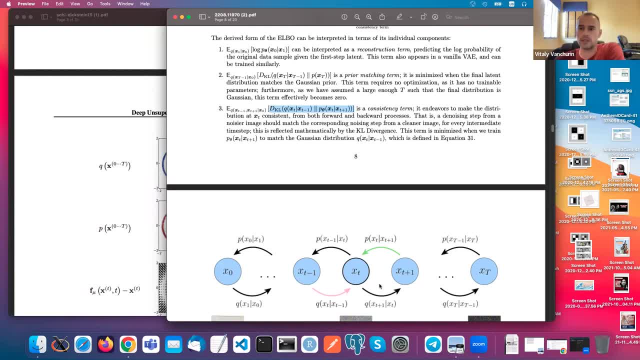 Have Few Parameters, Very Few Parameters, And Yet Gets From The Coherent Picture To Something Completely Random In The Long Number Of Steps, And That 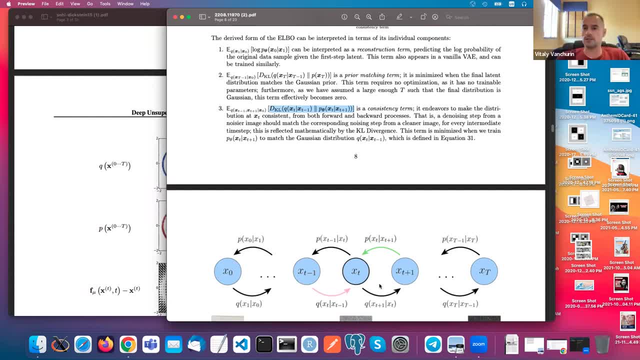 Makes The Covariance That We Discussed, And This Covariance Matrix Can Be Arbitrary. And What Are The Advantages, Disadvantages, Of Different Kernels? 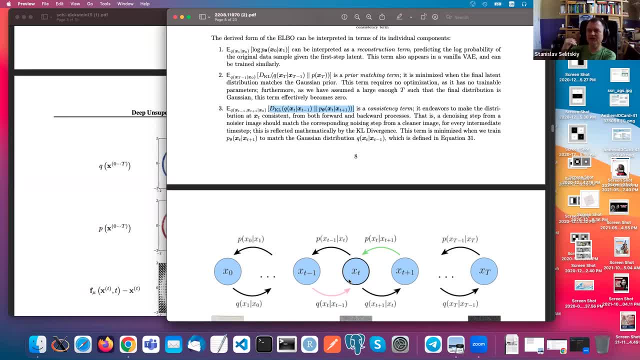 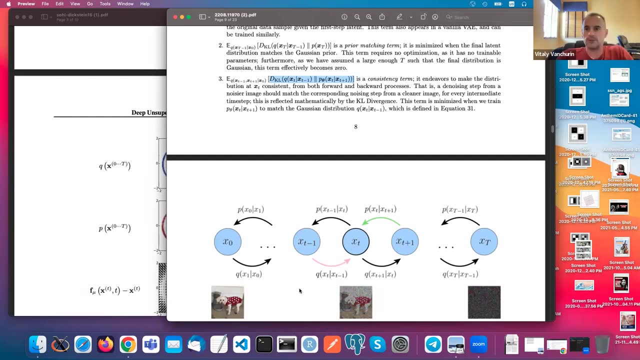 Now I Guess The Advantage Because, Like By Gaussian Steps, Yeah, The Fewer Parameters Easier To Train. No, I Understand It, But Again, Some Maybe 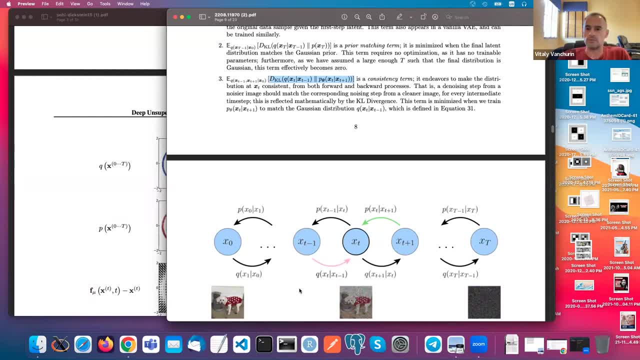 Theoretical Question Is Missing. Why Is This Or Not Some Other Kernel? It's Yes, Like Again. It's Like Again, Like Something Like Looking Keys. 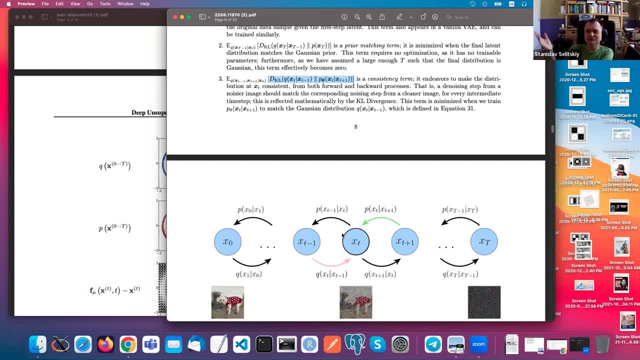 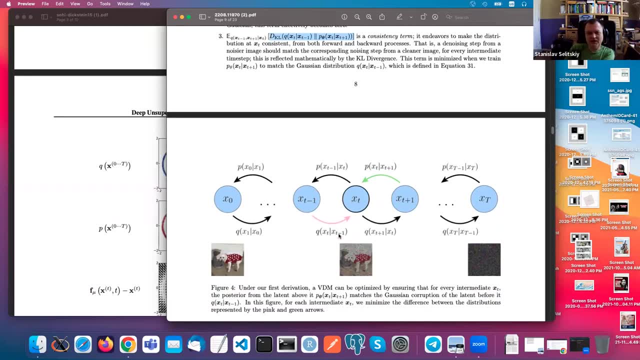 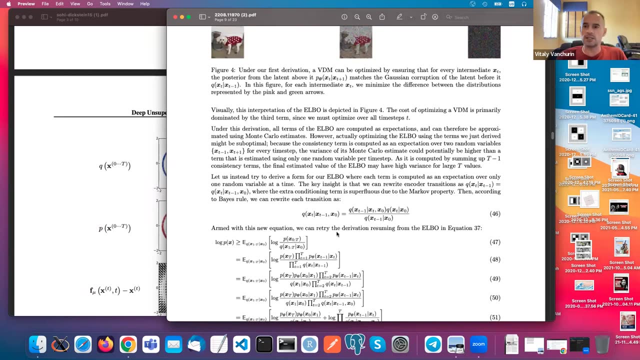 Under The Like Streetlight, Like It's Easy To Work Right Like Any Other Kernel, Like I Think. Let's Think About All Possible Transition Matrices. 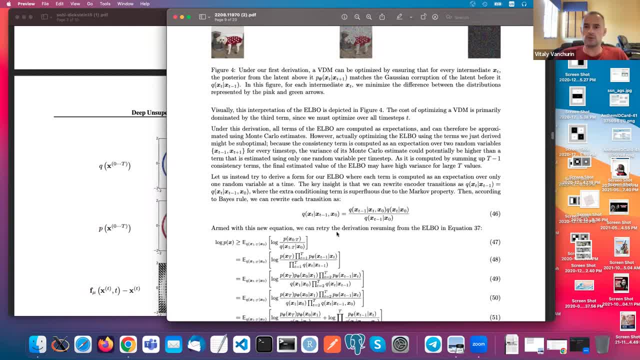 From You Know, Going To The Right Which You Describe This Conditional Queue, Right, This Is Conditional Distributions And, Yes, You Model Can And It. 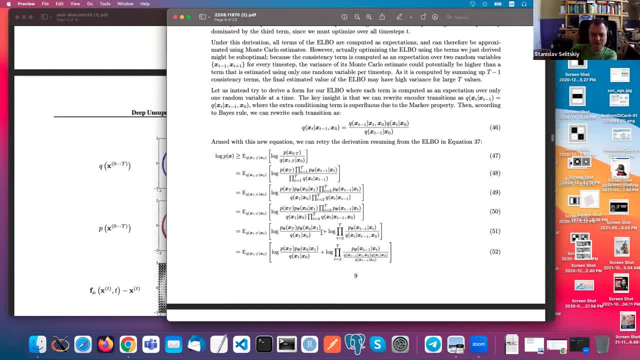 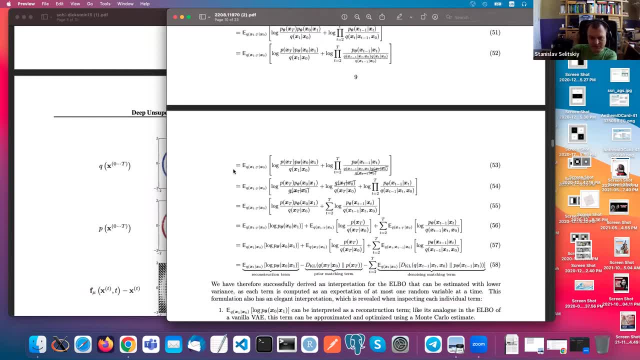 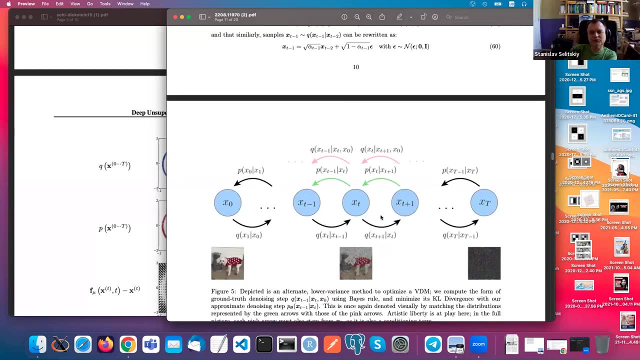 Works. Yeah, That Looks Like This Is The Reason. So Like Again, They Trying To Like To Massage Same Equations, Simplifying Steps, And Now They 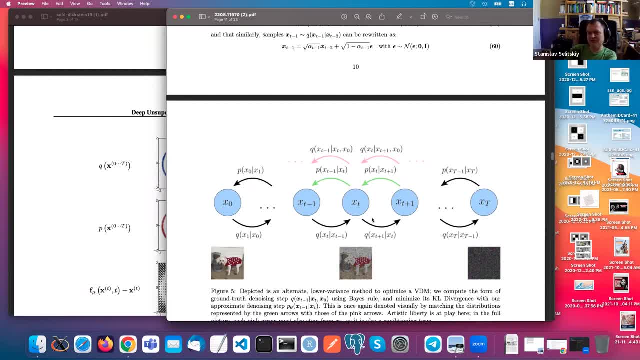 Yeah, This, This Is A Very Inverse Of Destruction. So Basically We Have Like Again, Like More theoretical. So We have This Theoretical Diffusion And 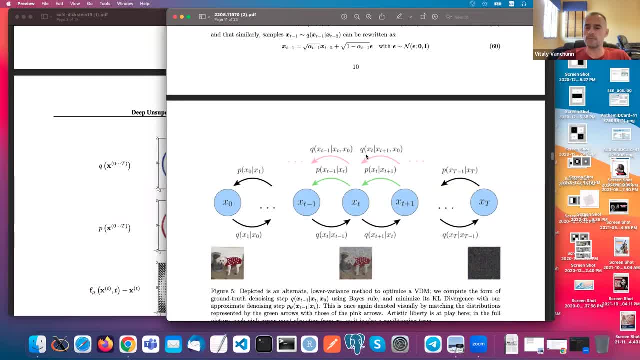 These Not Parametric, We Replace With Inverse Parametric. uh, i don't even understand why that works here, even if it did. um, because you know you cannot just write and set diffusion coefficient to be minus diffusion coefficient, uh, you will be getting something that makes no sense. they really like stressing a thing that we 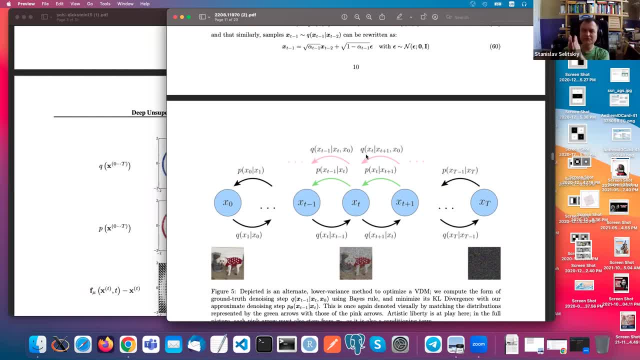 have really tiny, like, if you like, coefficients of diffusion and like in many steps, looks like this is still. i mean, you get like, basically what happens is like tiny uh fluctuation, like numerical instability, blows up. yeah, very small frequency modes, uh, high frequency modes, small scales for blow up. so that's why, yeah, looks like it would be like really interesting, like paper to 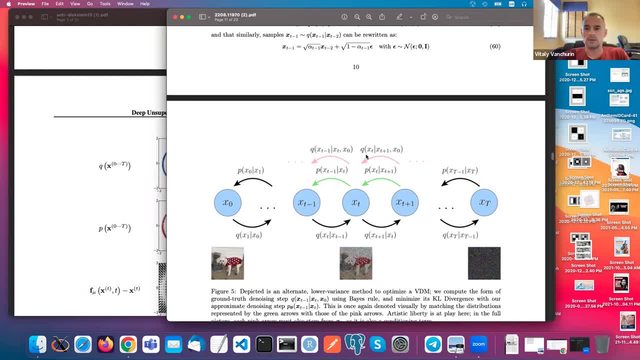 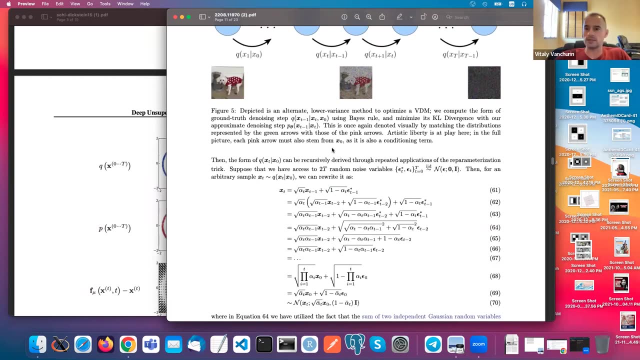 take this approach and right, like, blow it up and like show this is not very yeah like, uh, like generalizable sometimes might work. but so what you can do with anti-diffusion, it can like suppress uh, certain frequencies, like by hand, say, i do not allow like high frequencies to grow, and then you 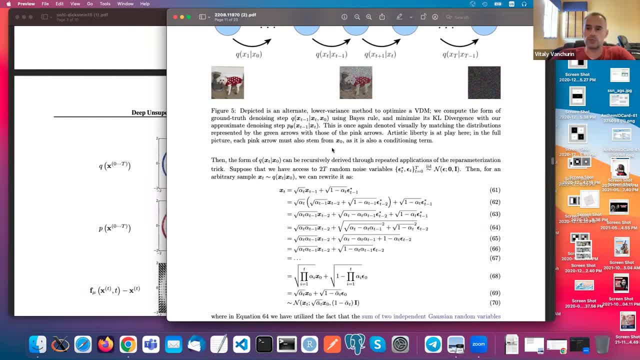 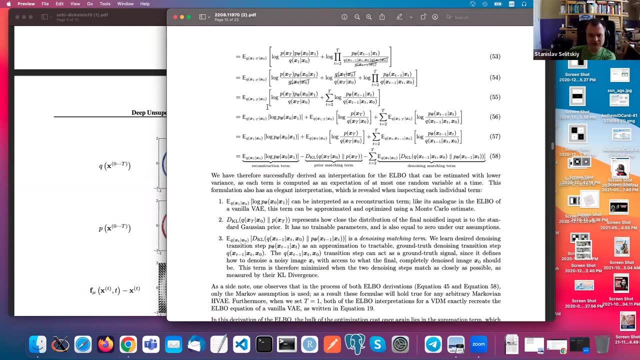 know by hand, regardless of what your diffusion equation, anti-diffusion equation tells you. you just suppress that. but but that, uh, yeah, okay, go ahead, sorry, yeah, yeah, uh, and uh like from here like more like generic, uh like equations when they map our like you, uh, uh, like 2p. 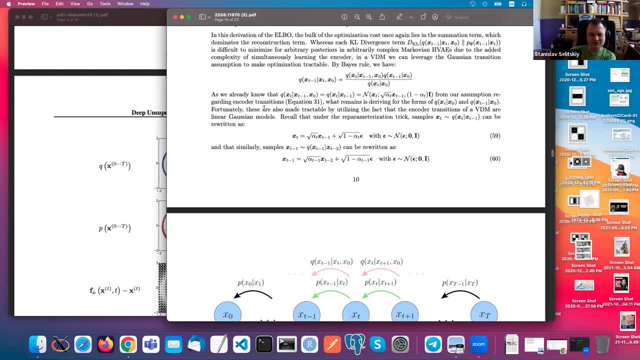 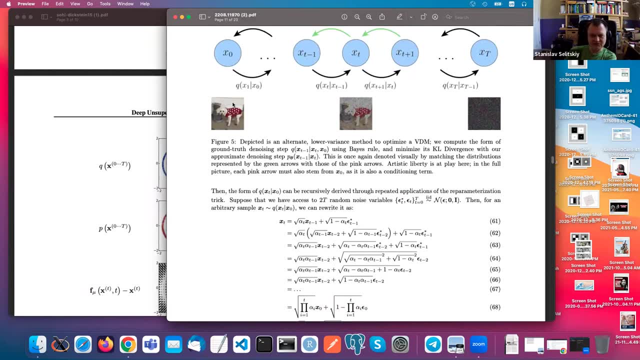 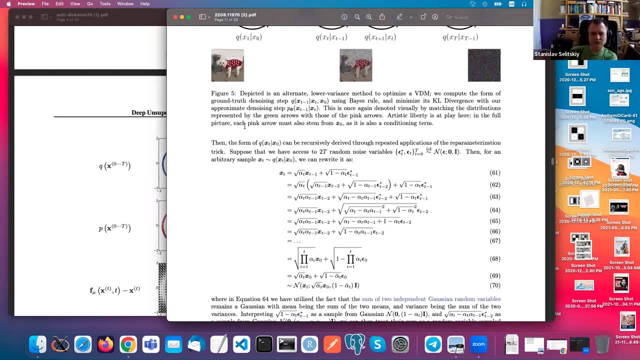 they come like again like a little bit, like complicated- uh, not complicated, but like tedious, like derivation. they come to like again like using optimization, using all these alphas which are like efficient, like on theoretical level- yeah, like you have to like really like to derive it and implement, like probably this is like level, like i stop understanding. 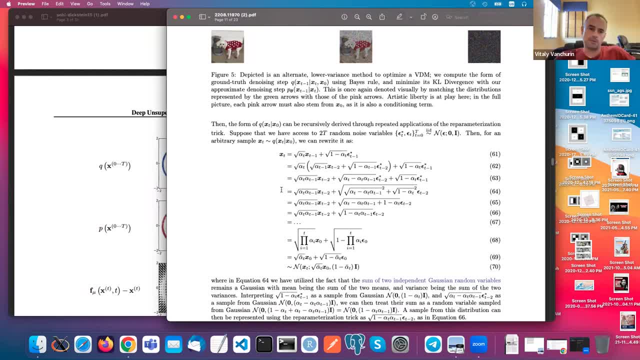 well, if it's the same mark of uh, a mark of uh matrix, that you multiply in each step, then it's very easy for you to know where you're gonna get. um, you just do the eigenvalue decomposition, this, you know, stochastic matrix, uh, and that's it. just like you solve like shortening equation for. 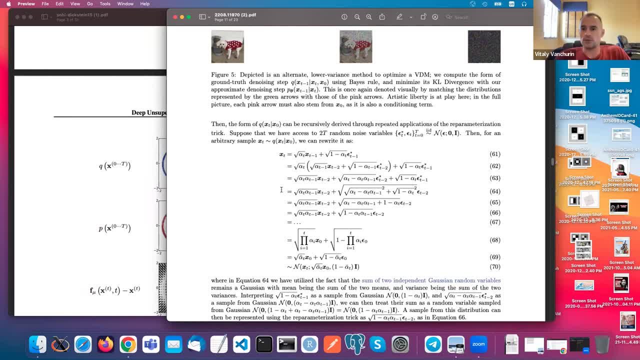 all the time you do the same. you take initial state, you will project it to the eigen eigen space of that matrix and then you will know exactly where it will end up. so this forward path is is relatively simple. uh, with a backward pass i'm not so. or or what they call reverse path, i'm. 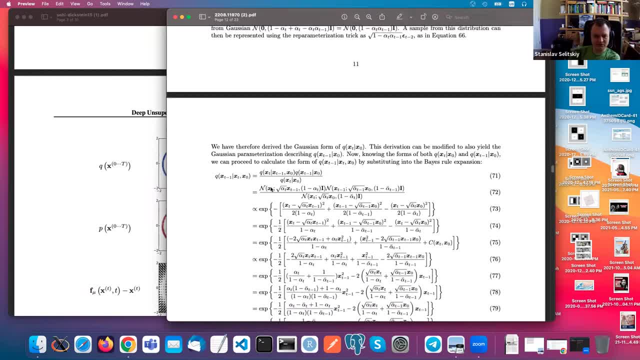 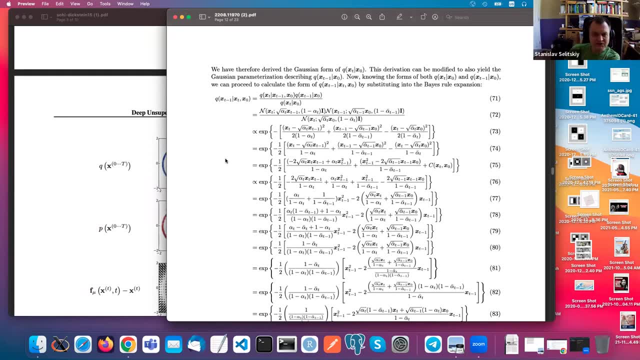 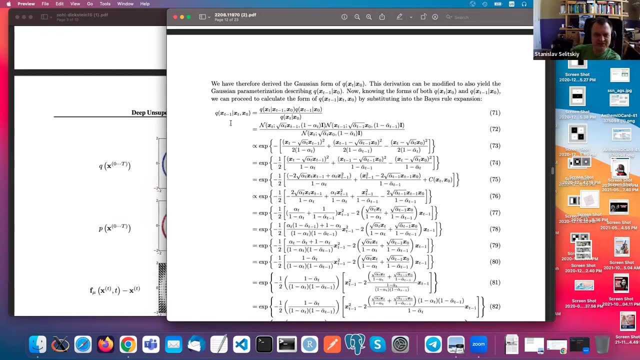 not so, yeah, reverse pass, but i think this is uh like what data i'm. so we have this like you, uh, and yeah, so, yeah, that's uh too complicated. yeah, yeah, yeah, and, and this is, i think this is uh like exactly so we have this not the forward cube, but, uh, our like like backward. 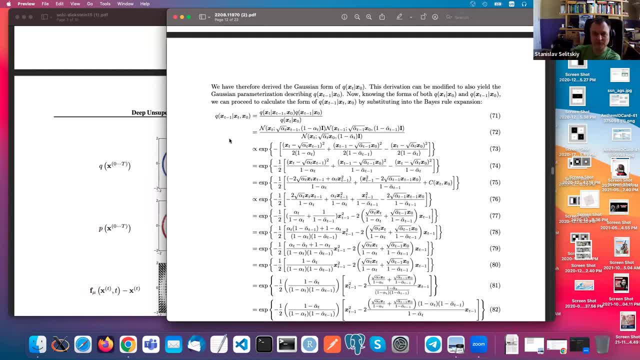 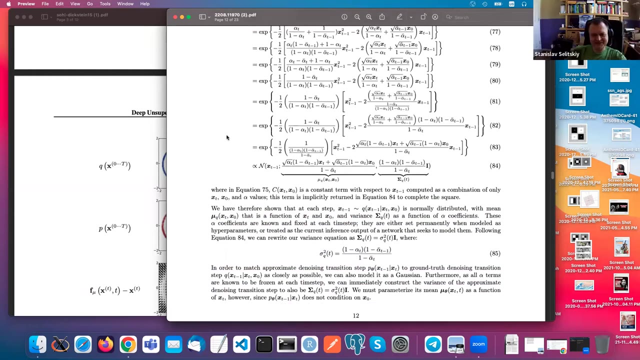 um, approximation of the cubicles, like we have this like t, like t minus one, so like period step, like conditioned on uh, uh, like on deeper one and uh on original state. so it looks like approximation of the p. but yeah, this, this is just too much. i think this is yeah. so yeah, that's too complicated. 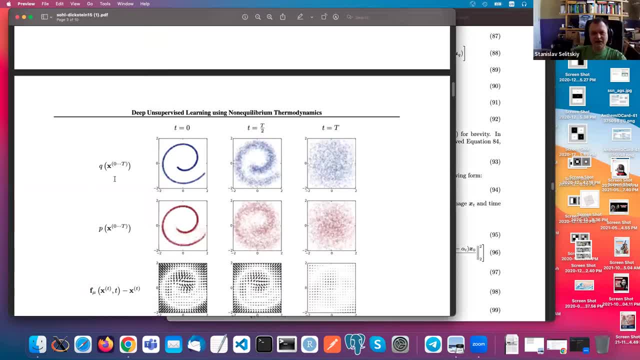 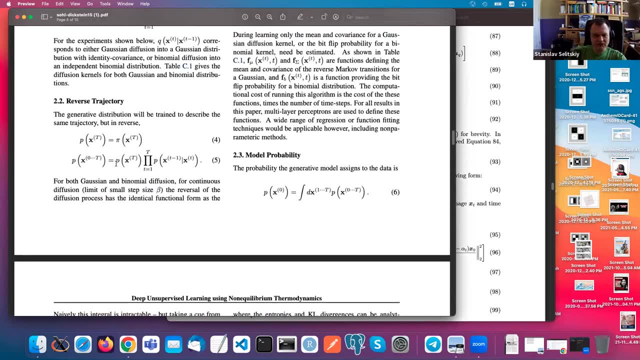 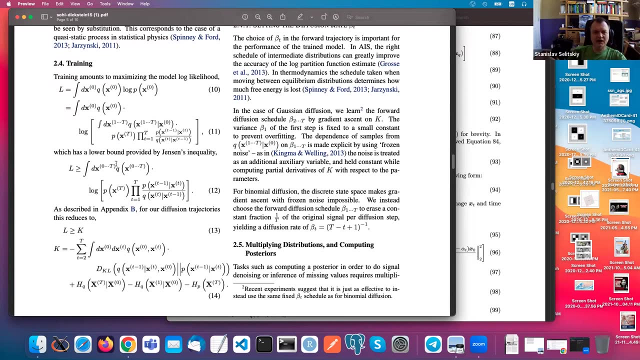 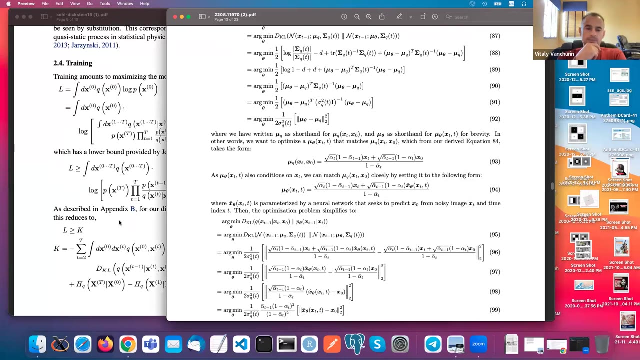 they cannot be right. yeah, yeah, yeah, so like uh, but anyway, so they uh in this original paper they uh. so basically have similar uh derivation and uh. there is also appendix, but it's less informative than this one, but if it's, it's easy to find. uh. what interesting what they show. 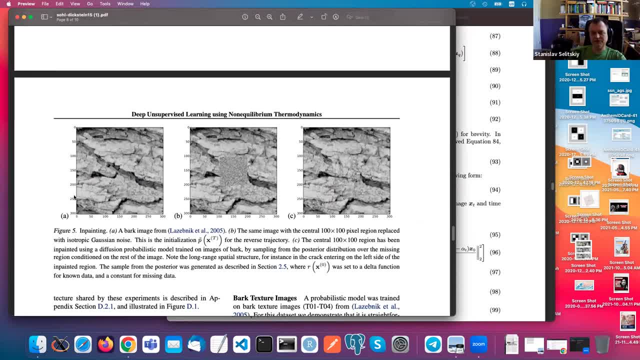 here practical application. so they have original image, uh, they uh want to. so they take this- uh gaussian noise in the middle, and they apply the algorithm to this fragment of the image on forward pass, they map it to gaussian and then they are restored to this way. so it's not. it's not exactly like original one, but which looks like similar. 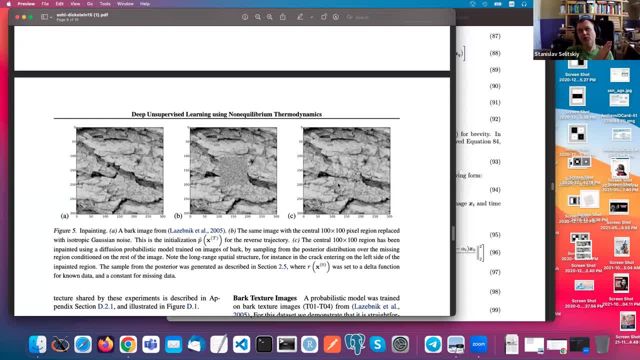 So it looks like when we map our original not parametric strange distribution to Gaussian in the bottleneck, like we reconstruct, like we probably map our not parametric again to something more theoretical. So basically we might create images in the middle, I guess. 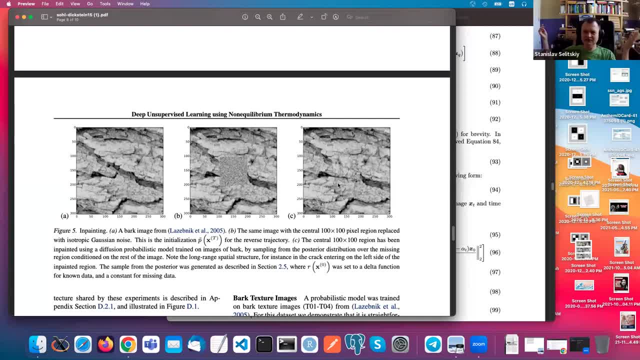 So this is some kind of stable diffusion image generation. So we have images of the big wave, images of the cats, And in the middle we create these images of both ways, like in cats, and more or less reasonable. Well for that. 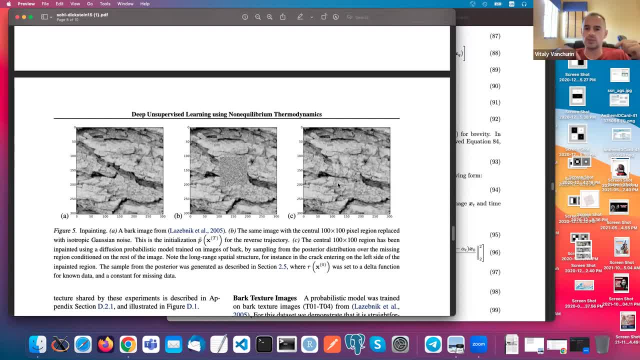 You also have to make sure that pixels on the boundaries are not diffused, because you would want to glue your new picture to the- you know, this interior square. You want to make sure that the boundaries of this are smoothly interpolated somehow, And so your diffusion should not probably have like smaller diffusion coefficient at the boundaries or something like that. 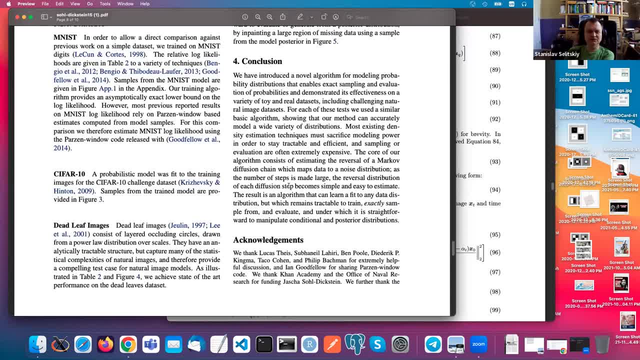 But yeah, And this is like original, I think this is like 2015.. Mm, hmm, Mm, hmm. So since then, you know it was like a lot of progress, So we'll have to understand what the progress was. 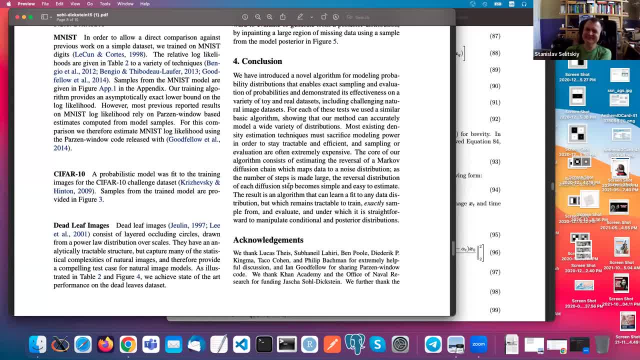 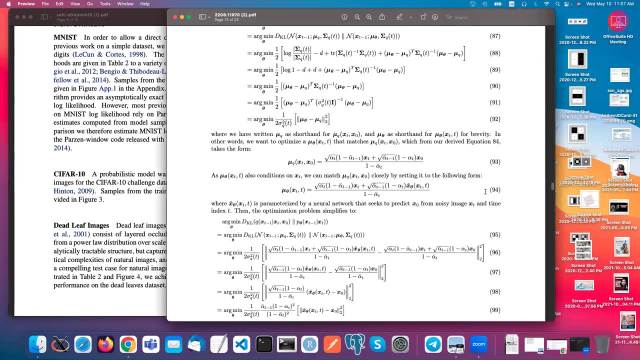 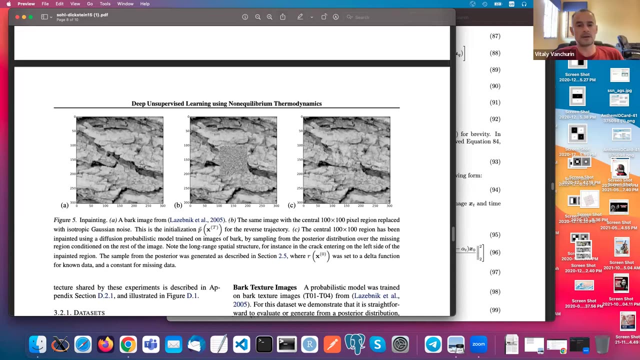 Yes, Yeah, Okay, So this probably is like what I was able to like to get intuition for this. Okay, Any questions? Yeah, Quick question. So the picture you just showed, the figure with the Gaussian noise and the filter- Is that so? is that due to diffusion in the model or like, like what are they trying to show here specifically, like that just the model can do it, because I'm pretty sure, like without diffusion, something like this could also be done. 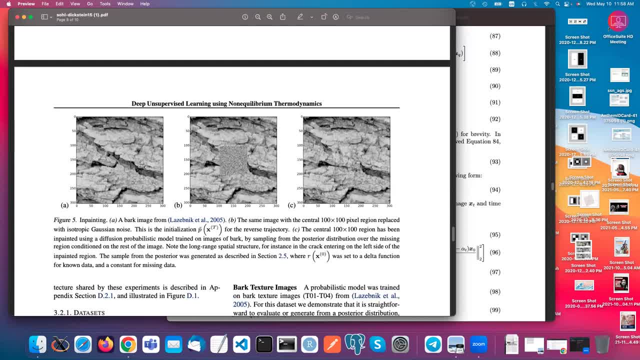 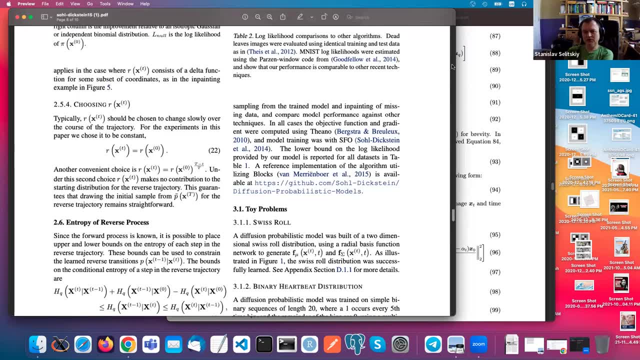 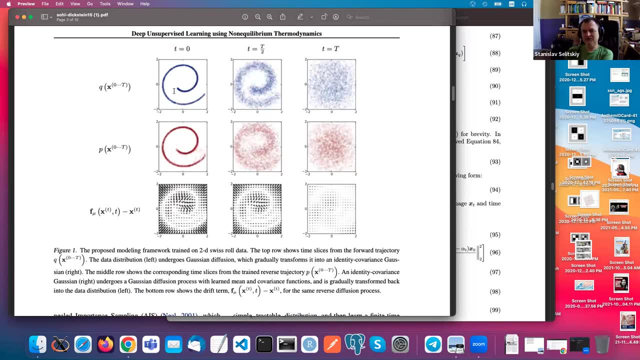 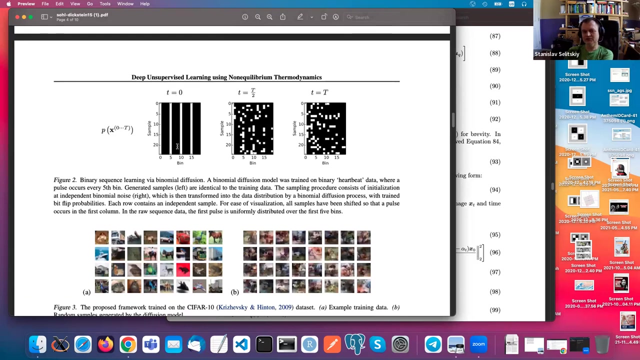 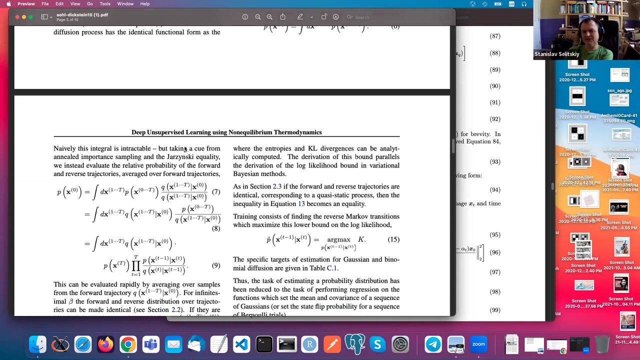 So I guess my question is like: what is the advantage of diffusion? I'm still kind of lost on that. I guess they just introduced like this: This method is one of the first papers And they Use like completely like toy, like problems, like here. then we have the Swiss roll. we can diffuse it and reconstruct something like wishes, like looks like original. they use another like toy problem, like we have this heartbeats, like like pseudo heartbeat things and like we diffuse it and and reconstruct and they are the like demonstration what we can do with this. 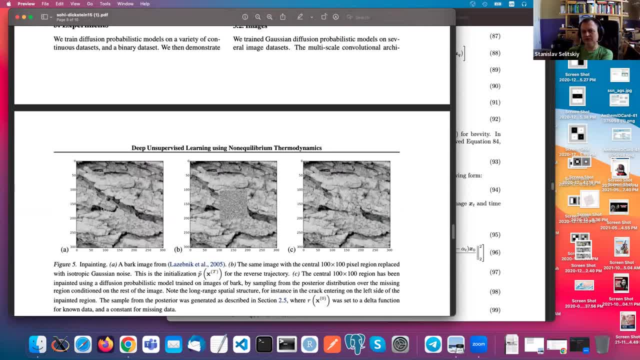 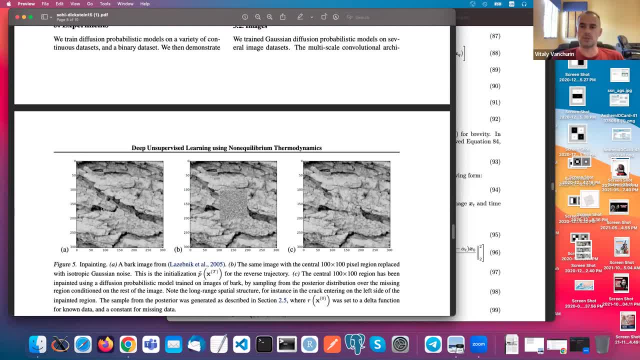 I think Vladimir's question was just like mine: you know what's, what is it good for? So, but maybe is it because it uses fewer parameters it's faster to learn train. Yeah, So in the paper, in this, in this paper, they do like have four bullet points on, like the. 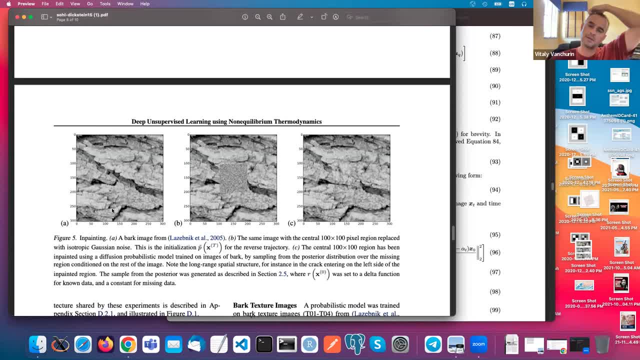 advantage of their model, but it doesn't seem like they explicitly state that it's due to diffusion. So I'm not too familiar with these models, so that's why I'm kind of lost. but maybe it's these points like easy multiplication. 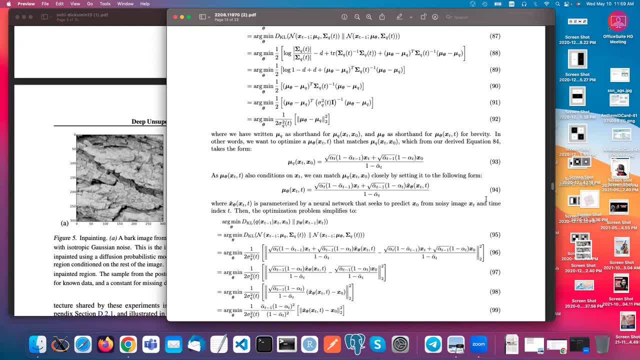 with our distributions, although I think that's not really due to diffusion. Yeah, exactly, But diffusion can be permitted by a few parameters, so maybe that's kind of-. Yeah, well, it seems like it's also like a regularization approach. 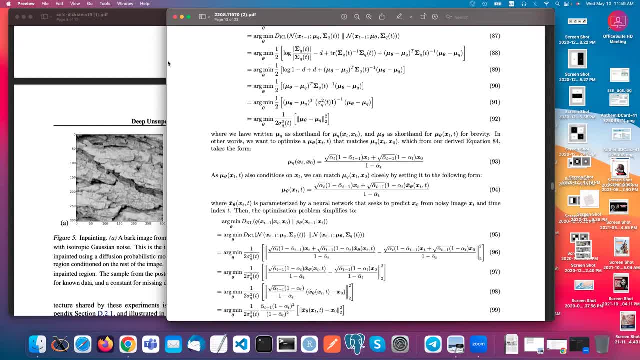 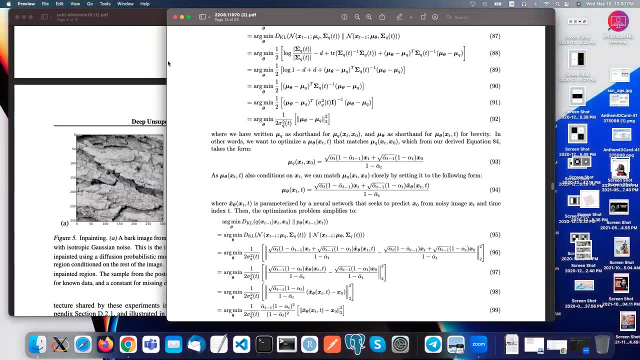 It's like an alternative regularization. like you have dropout, you have other approaches to regularize. this is like another one, But then I would expect them to like compare it to other models where they have other regularization or no regularization, which it doesn't seem like. 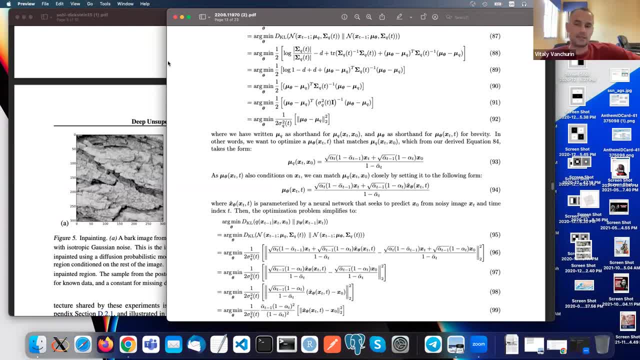 they do that here either. so, Yeah, I agree. This is- that was my question- like: what is it good for? Yeah, good for us, Yeah. so yeah, looks like they just. oh, this works and yeah. 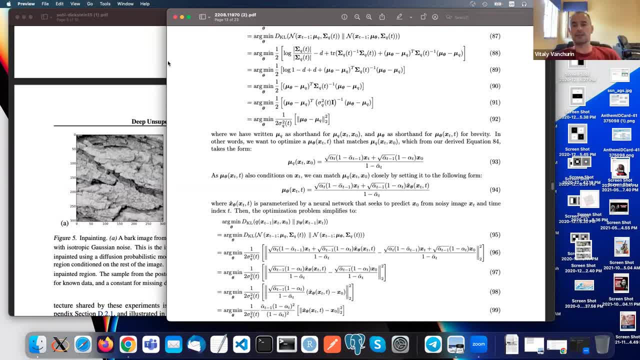 No, but you do want to have a comparison. say, here it is. you know, we have fewer parameters and it works as good as with the dropout players, or whatever it is. Yeah in the second, yeah in the second paper. they-. 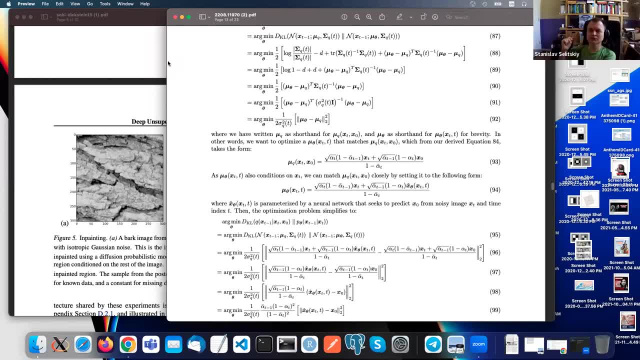 They do that. okay. Yeah, they still like don't compare, but they highlight this like stroke points. so we have this like tractable analytic, like equations and we can train fast and easy. then Well, tractable analytic equations is good for right. 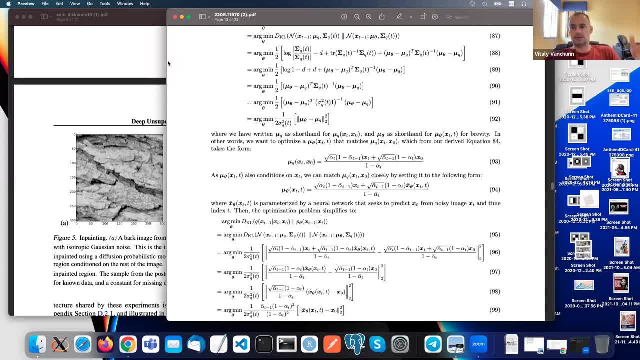 Writing equations. but when it comes to the you know practice, right. if you're claiming the diffusion model is better than everything else, then you should really say why is it better from you know, development point of view application.